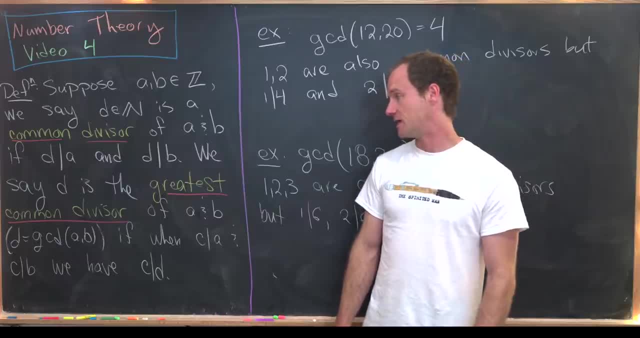 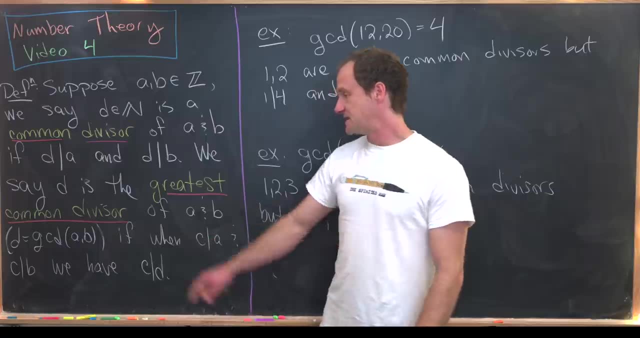 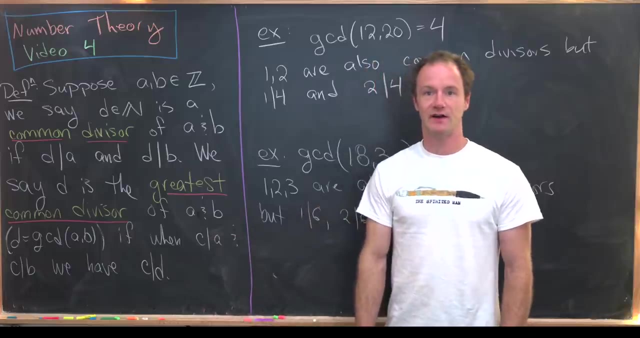 d is the greatest common divisor of a and b And we'll write: d equals gcdab. if when c divides a and c divides b, we know that c divides d. So other words, if we've got another common divisor, C, C must divide that greatest common divisor. 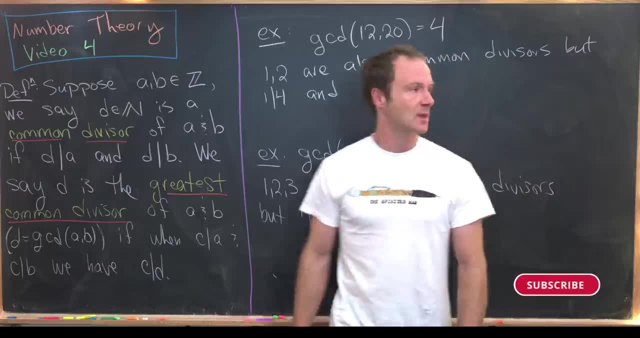 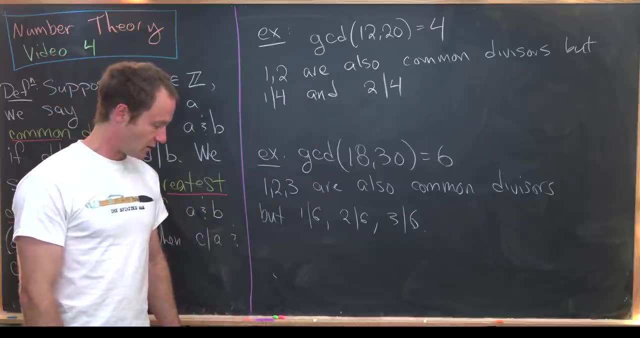 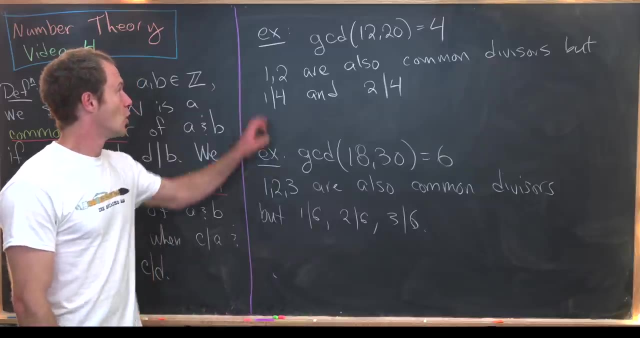 So our ordering here is like by divisibility. Okay, so two quick examples before we start proving things. First off, the GCD of 12 and 20 is 4. And so you can see that just by kind of elementary school arithmetic. 1 and 2 are also common divisors, but 1 divides 4 and 2 divides 4.. 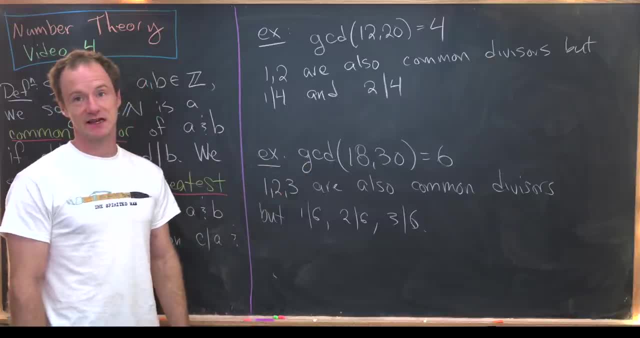 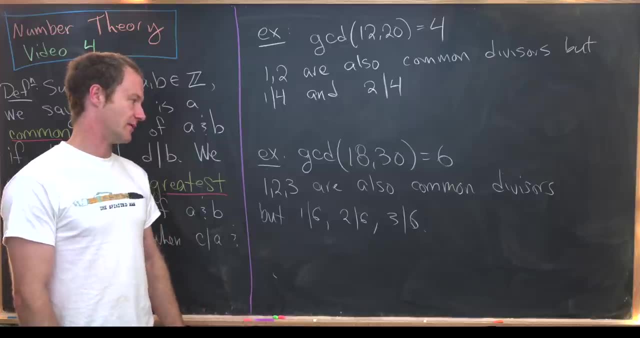 Next, the GCD of 18 and 30 is 6.. So again by elementary school arithmetic we know that 1,, 2, and 3 are also common divisors, but 1 divides 6,, 2 divides 6, and 3 divides 6.. 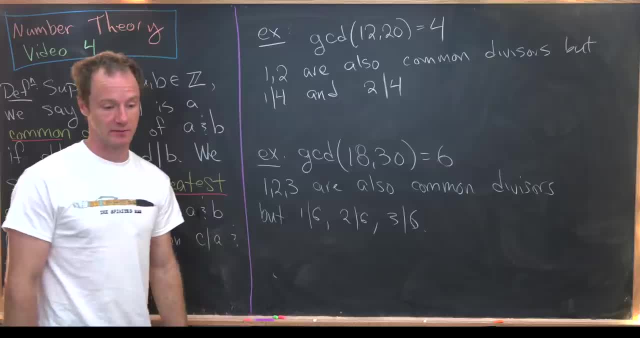 So you can play this game all day long with small numbers, but eventually we'll get to the point where we're going to get to the point where we're going to have to make sure that there's a common divisor. So let's start by putting in a good number of primary. 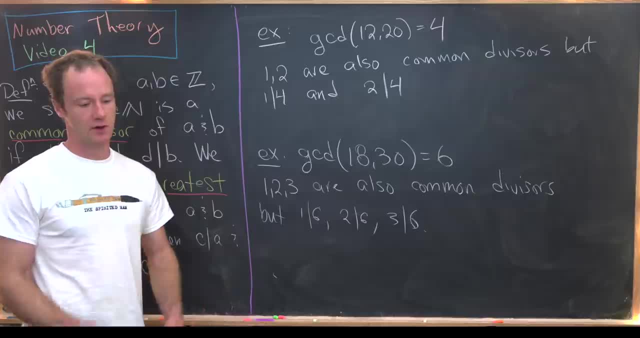 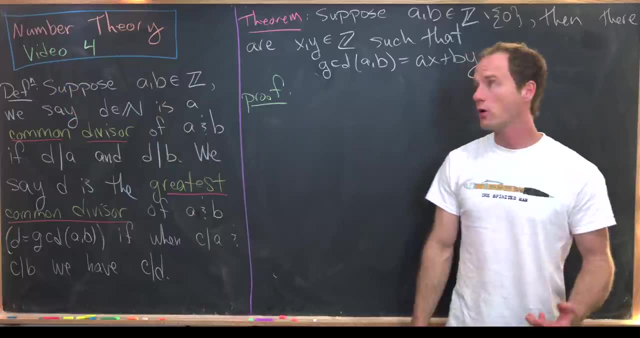 need some sort of method for finding the greatest common divisor of larger numbers. That's actually something we're working towards, Okay, so let's get rid of this and we'll look at our first result. Okay, so the first theorem that we want to look at is about writing the gcd of two integers as: 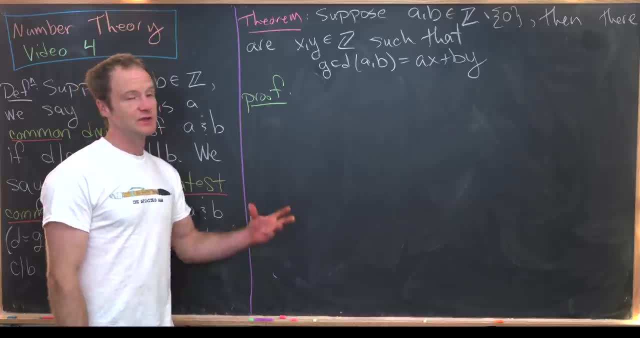 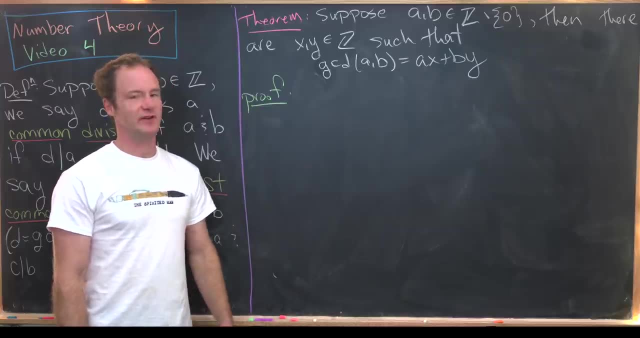 a linear combination of those two integers. So let's start by supposing we have non-zero integers a and b. You could extend this to having one of them be zero, but it's not super interesting. Then there are integers x and y, such that the gcd of a and b is equal to ax plus. 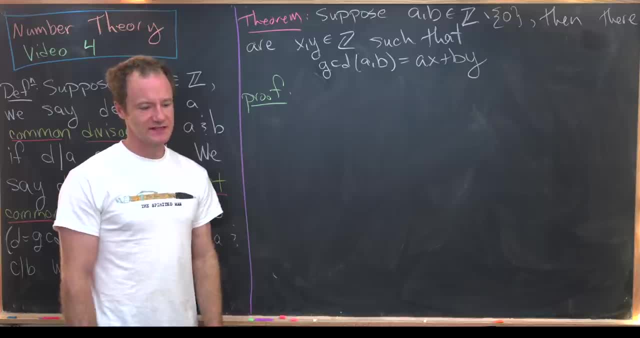 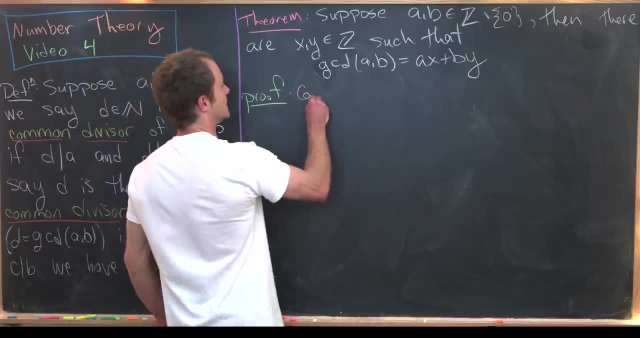 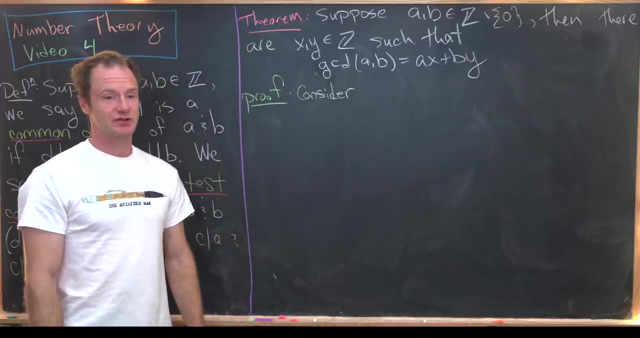 by Okay, so let's maybe see how this proof goes. And this proof uses a similar technique to what we saw with the division algorithm, So we're going to consider some sort of set and then use properties of the natural numbers in order to get something. 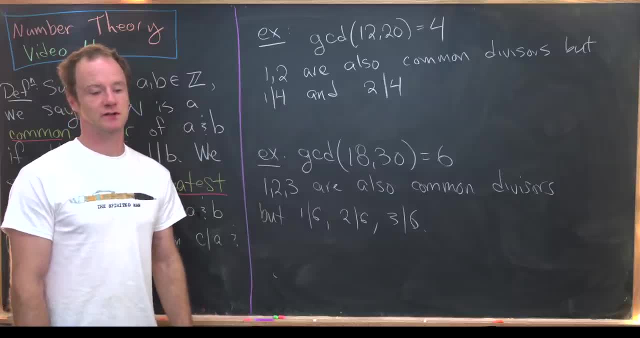 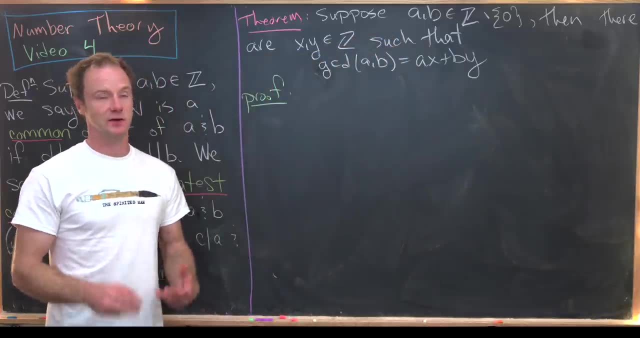 Okay, so let's get rid of this and we'll look at our first result. Okay, so the first theorem that we want to look at is about writing the gcd of two integers as a linear combination of those two integers. So let's start by supposing we have non-zero. 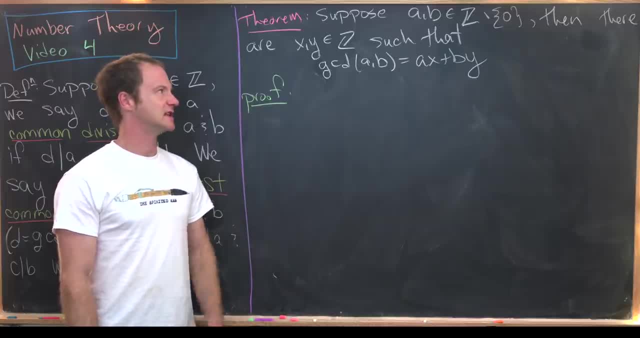 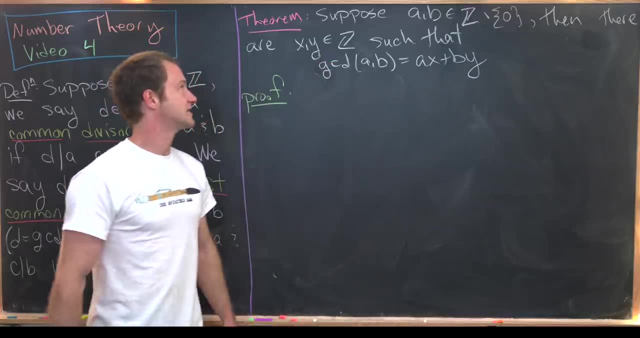 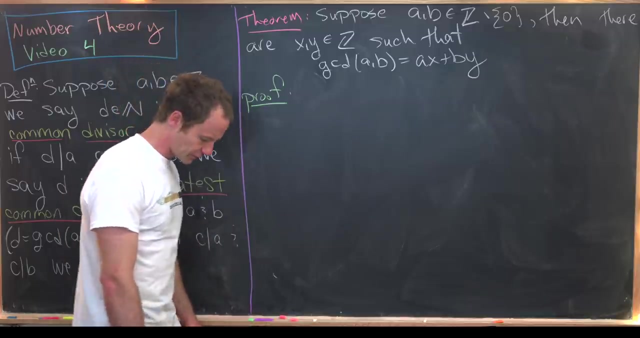 integers a and b. You could extend this to having one of them be 0,, but it's not super interesting. Then there are integers x and y, such that the gcd of a and b is equal to ax plus by Okay, so let's maybe see how this proof goes. And this proof uses a similar technique to 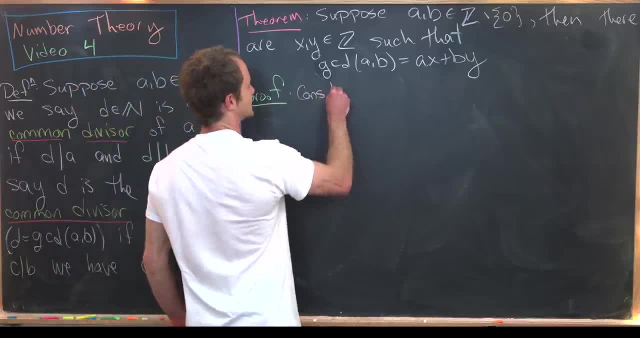 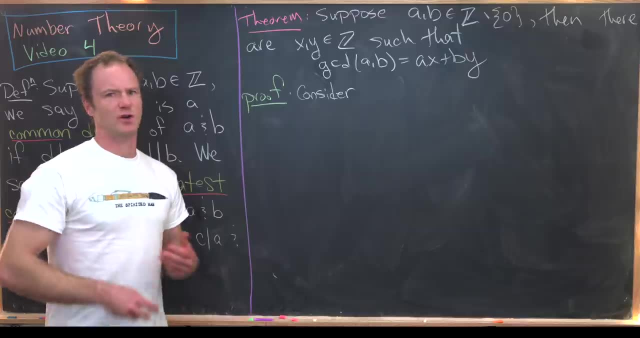 what we saw with the division algorithm. So we're going to consider some sort of set and then use properties of the natural numbers in order to get something out of that set. So here's what we'll do. We'll take this set, which I'll call a. 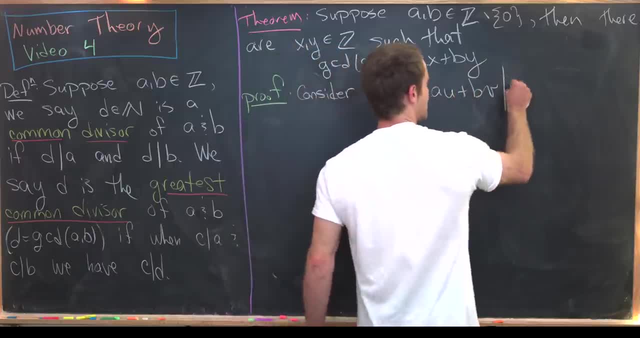 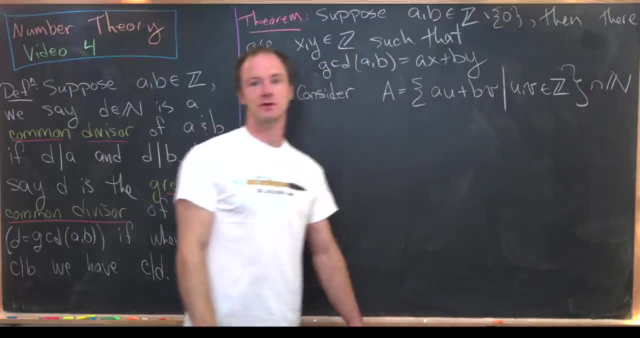 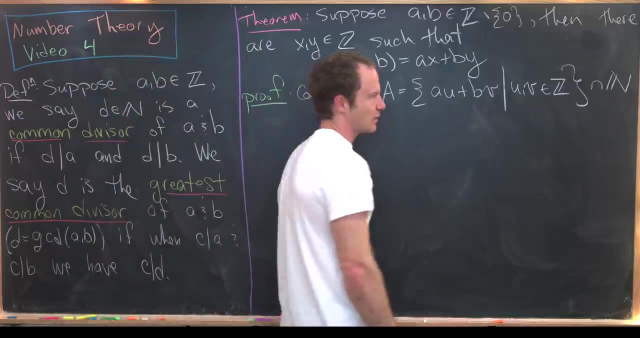 to be au plus bv, as u and v range over all integers, And then I'll intersect that with the natural numbers And I should say here I'm taking the natural numbers not to include 0.. So if you want to put like a star up here to say that we're just including the positive, 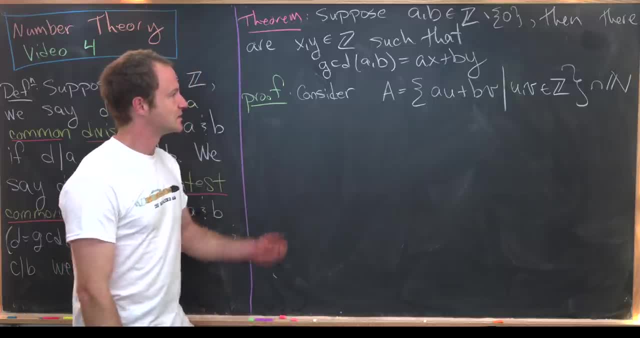 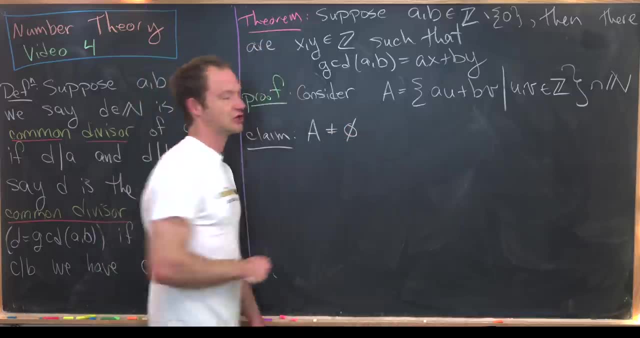 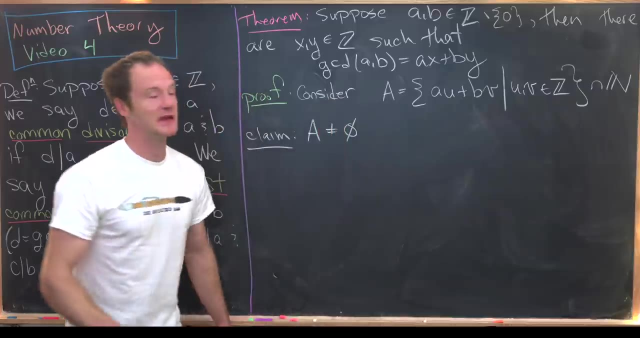 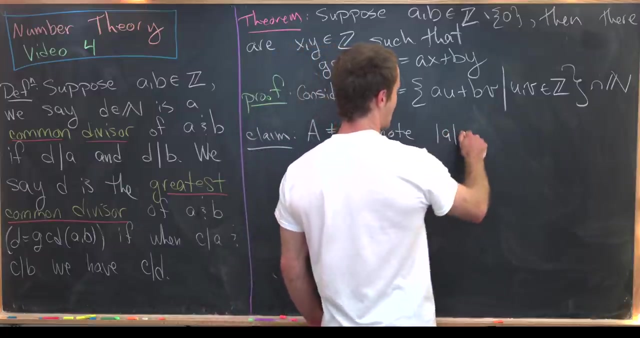 integers, then you can do that if you're psyched. Okay, so now my first little claim here is that my set a is not equal to the empty set. Now, how could we do that? Well, since a and b are both non-zero, notice that the absolute value of a is equal to plus or minus a, That's. 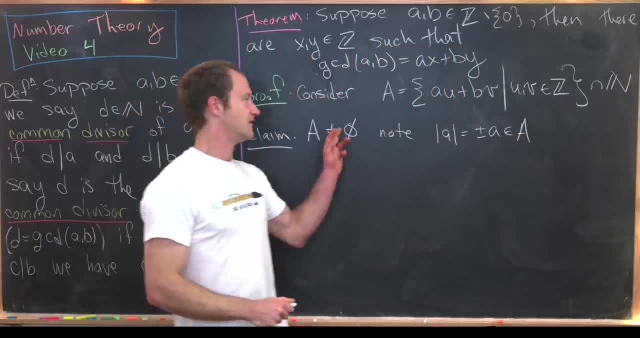 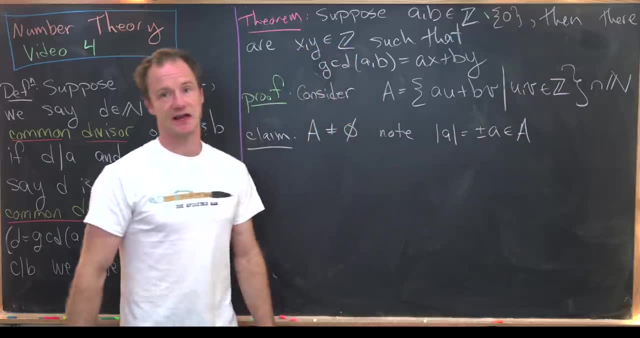 an element from a. Well, if a is negative, we'll just take negative a that makes it positive, That makes it a natural number. So it's in both of these sets, Just take u to be negative 1.. And then, similarly, the. 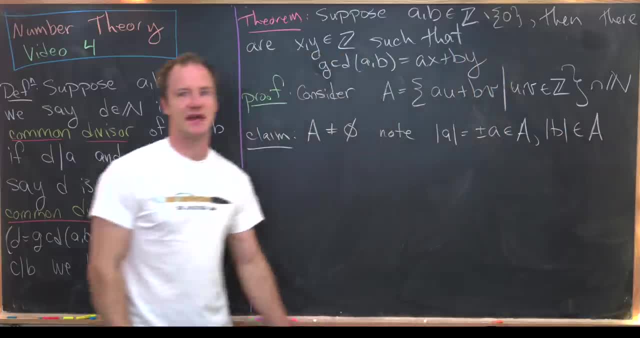 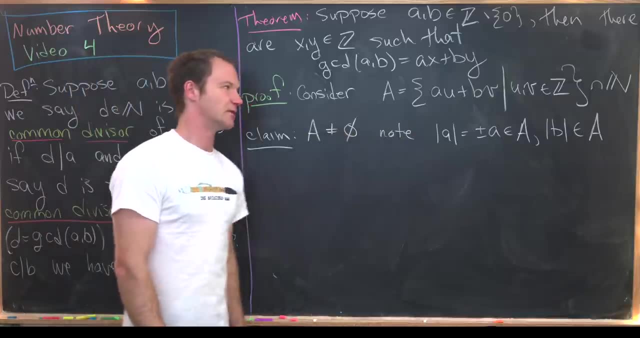 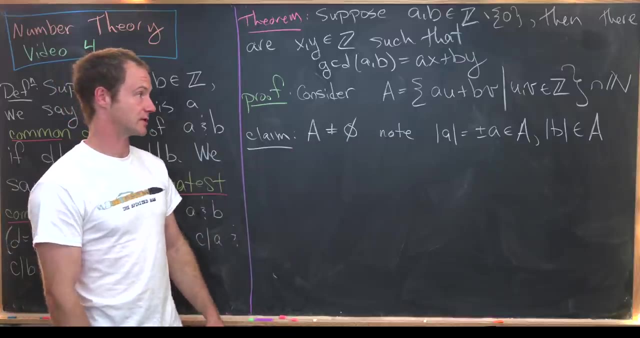 absolute value of b is in the set a. Now, if we only took one of those to be non-zero, then obviously you would take whichever one here is non-zero. Okay, so now that we've got a non-empty set of natural numbers, we know it's a set of natural numbers because 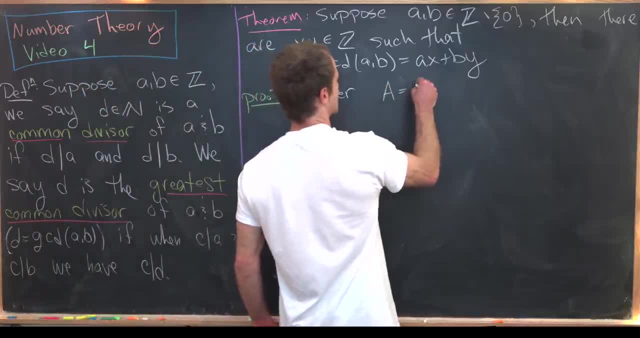 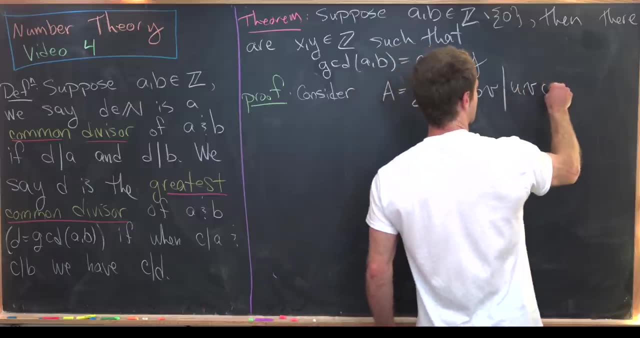 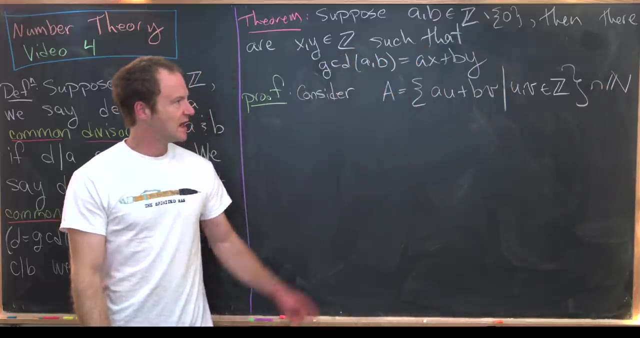 out of that set. So here's what we'll do: We'll take this set, which I'll call a, to be a, u plus b, v, as u and v range over all integers, and then I'll intersect that with the natural numbers And I should say here I'm taking the natural numbers not to include. 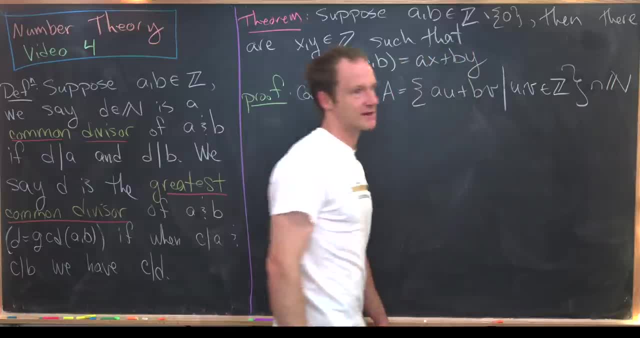 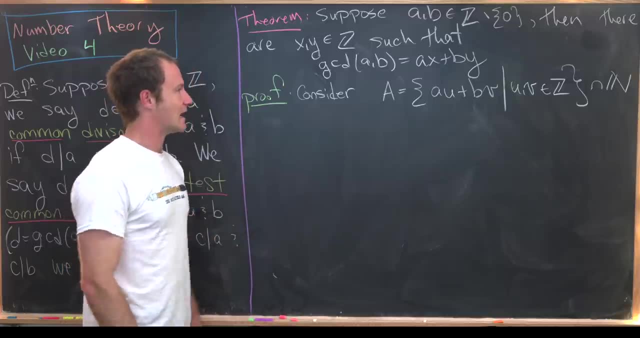 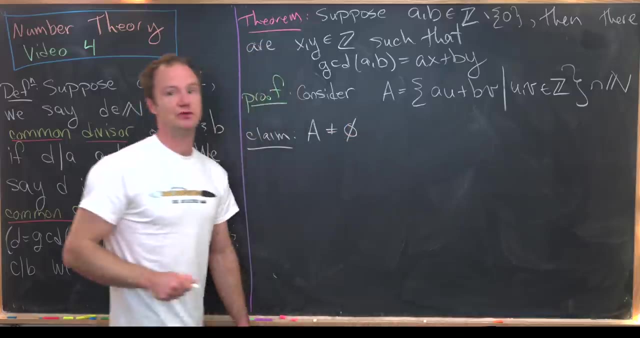 zero. So if you want to put like a star up here to say that we're just including the positive integers, then you can do that if you're psyched, Okay. so now my first little claim here is that my set a is not equal to the empty set. 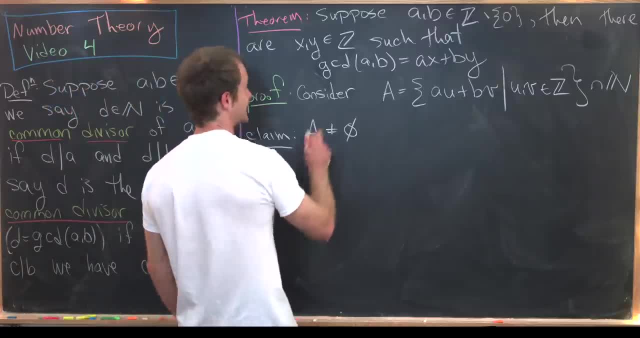 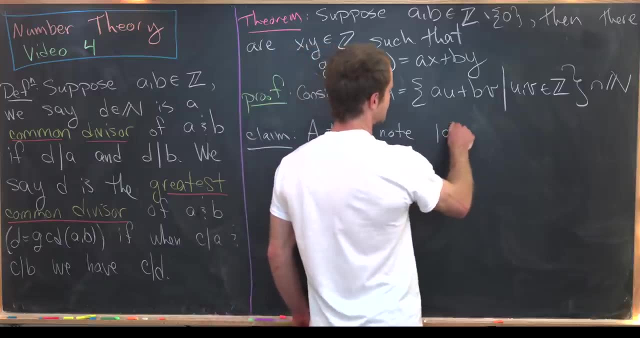 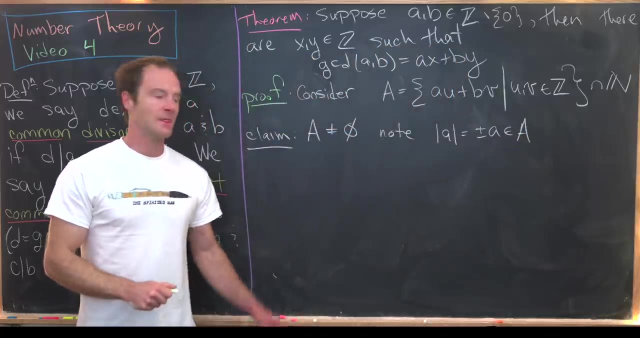 Now, how could we do that? Well, since a and b are both non-zero, notice that the absolute value of a is equal to plus or minus a. That's an element from a. Well, if a is negative, we'll just take negative a. That makes it positive, That makes it a natural number. 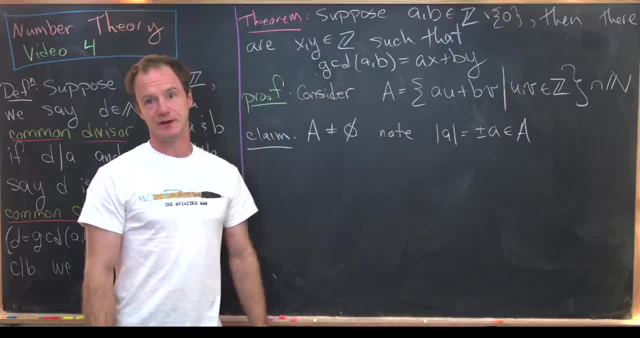 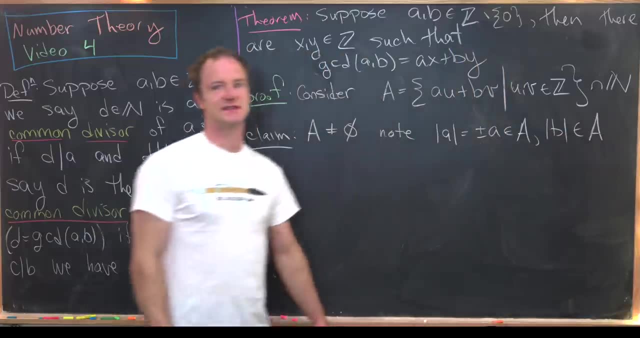 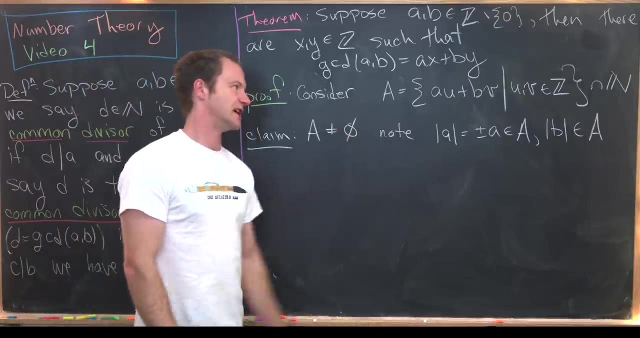 so it's in both of these sets. Just take u to be negative one And then, similarly, the absolute value of b is in the set a. Now, if we only took one of those to be non-zero, then obviously you would take whichever one here is non-zero, Okay. so now that we've got a non-empty. 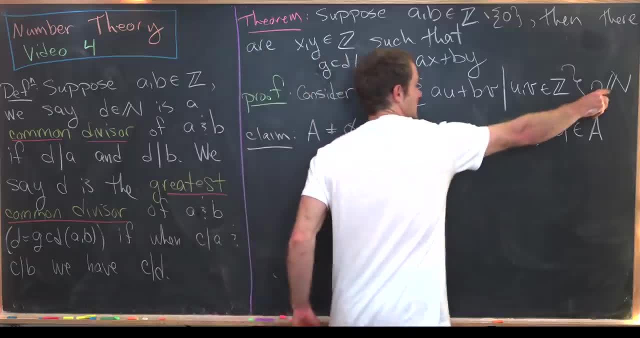 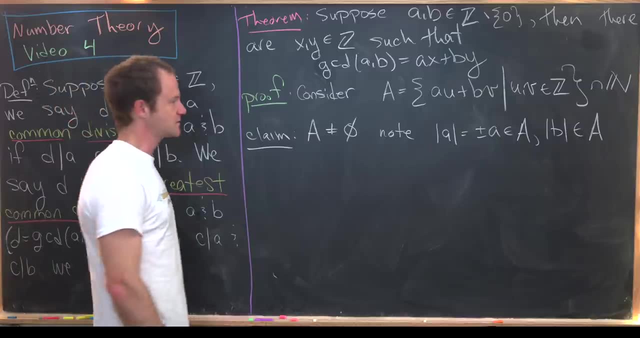 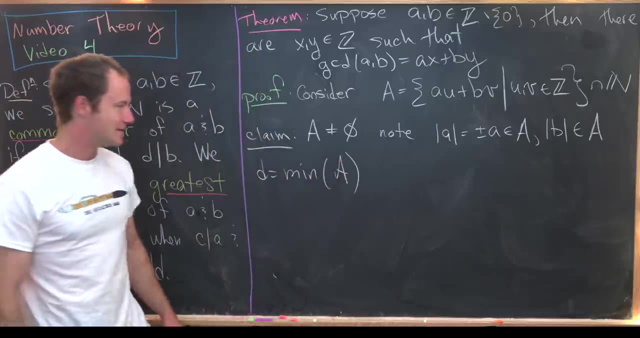 set of natural numbers. because of this intersection, it has a least element by the Archimedean Principle. So let's let d equal that least element. So I'll set d equal to the minimum of a. so let's just put here that we're doing this by the Archimedean Principle. 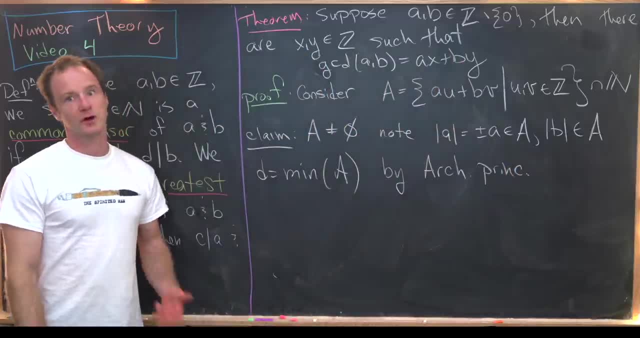 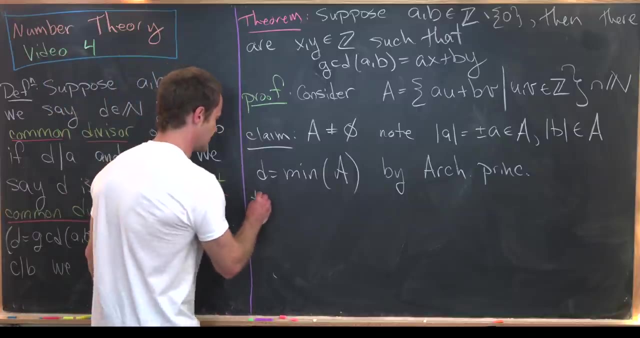 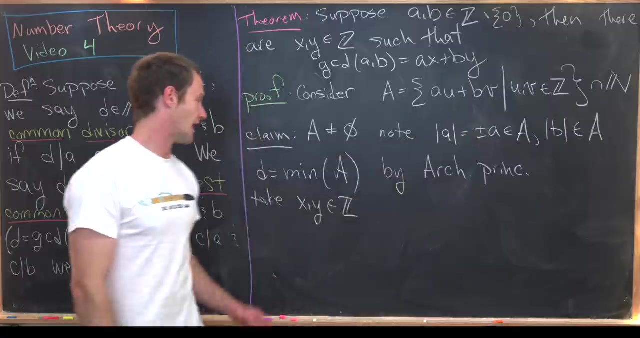 which says: or it's equivalent to every set of natural numbers having a smallest element, but now that d is of the form a, u plus b, v. so what we'll do is we'll take x and y integers to be the values of u and v that make this happen. so i'm just going to write this as such, that 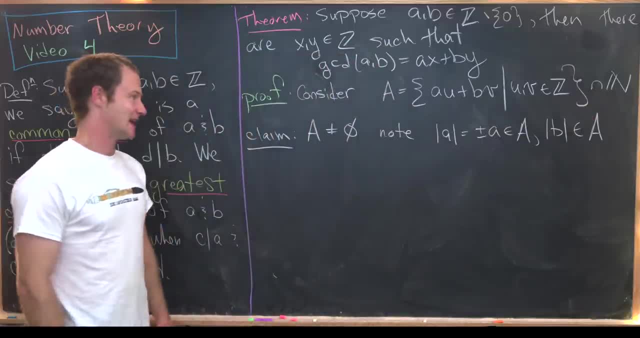 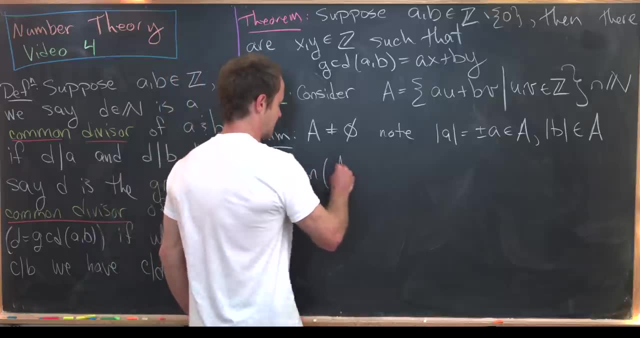 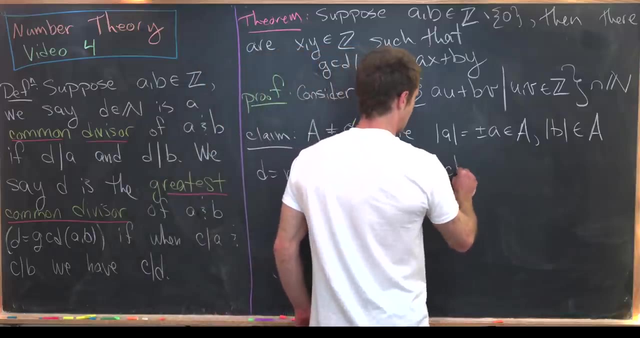 of this intersection. It has a least element by the Archimedean principle. So let's let d equal that least element. So I'll set d equal to the minimum of a. So let's just put here that we're doing this by the Archimedean principle, which says: or it's equivalent. 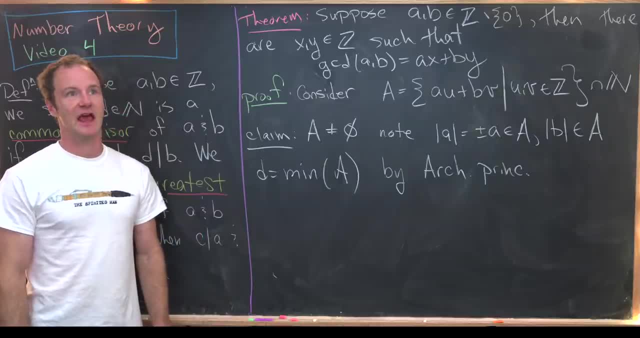 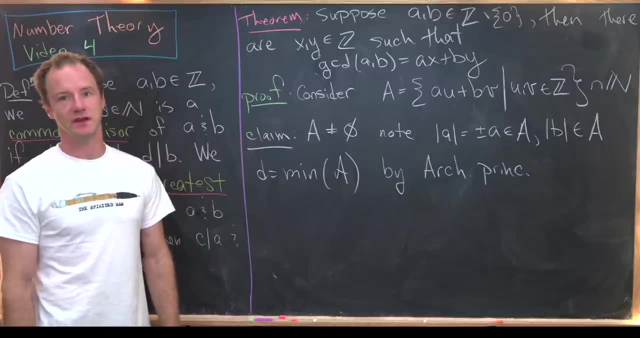 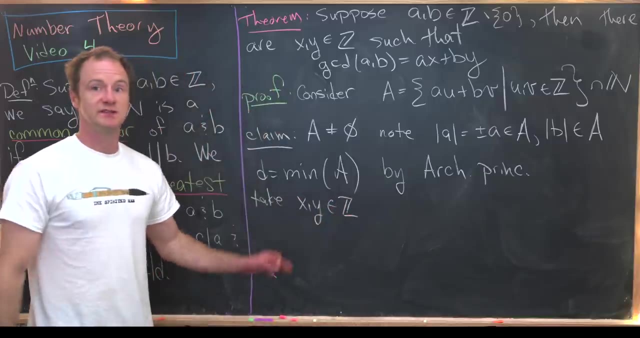 to every set of natural numbers having a smallest element. But now that d is of the form au plus bv. So what we'll do is we'll take x and y integers to be the values of u and v that make this happen. So I'm just going to write this as: 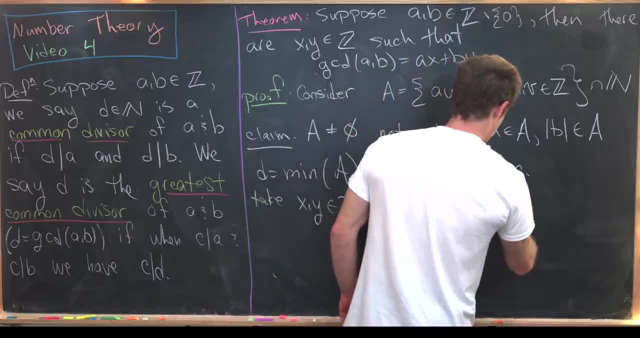 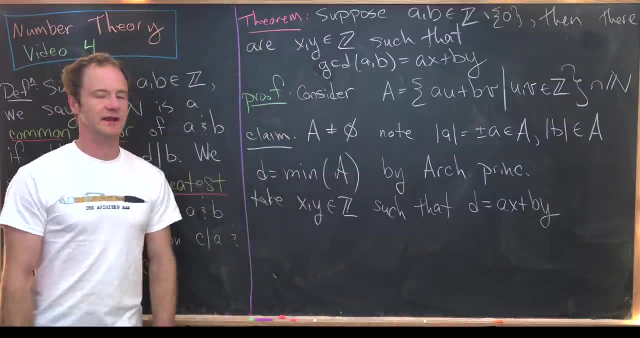 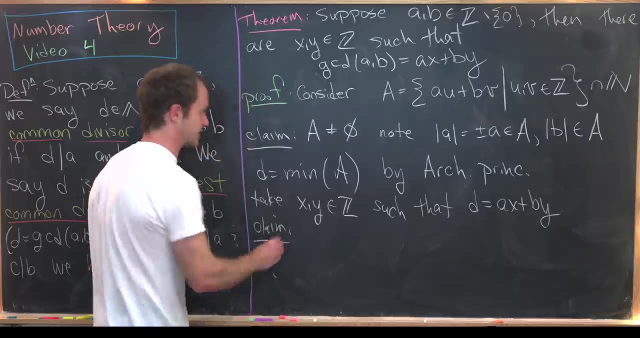 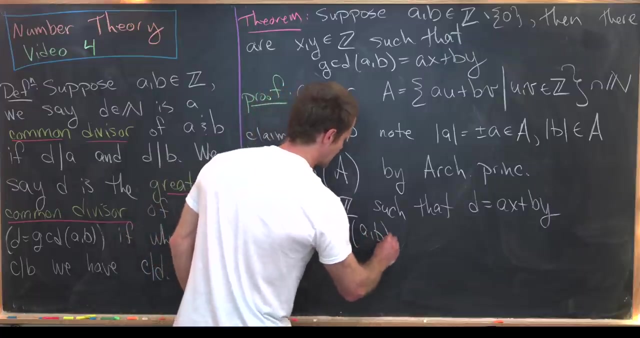 such that d equals ax plus by. Okay, but now look what we've got going on here. It looks like we're constructing it Exactly what we want, So that'll be our next claim is that we've actually constructed what we want. In other words, d is equal to the GCD of a and b, But we don't have room for. 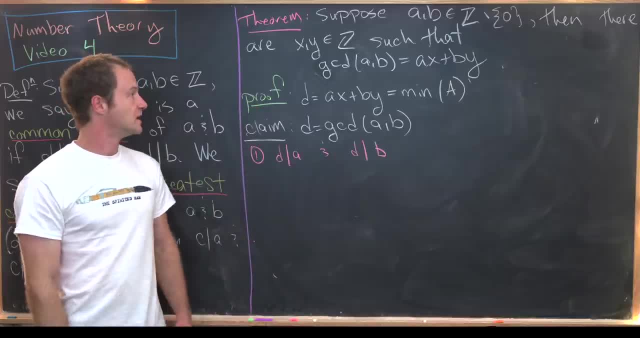 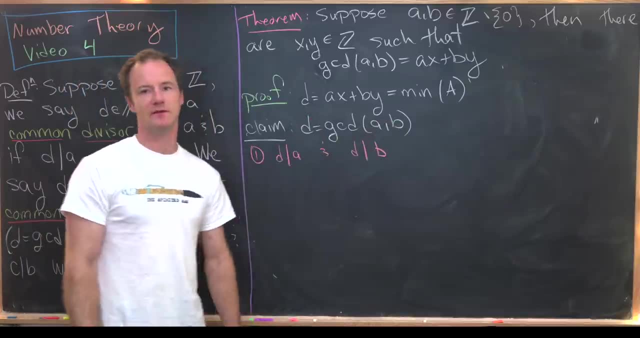 that here, So let's start over at the top. Okay, so on the last board we constructed this number d as a linear combination of a and b as the minimum of some set a which we had on the last board. Now I want to claim that d is the. 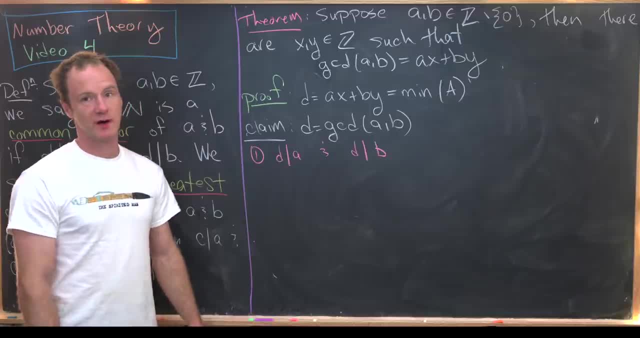 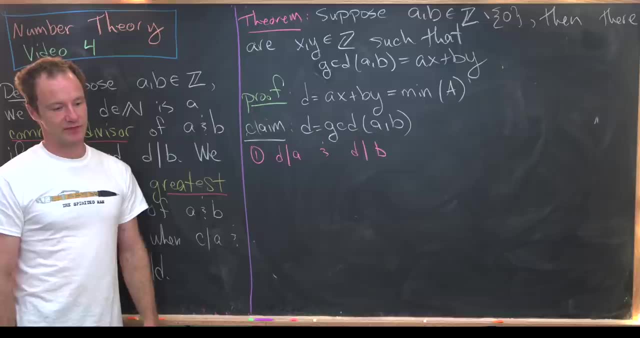 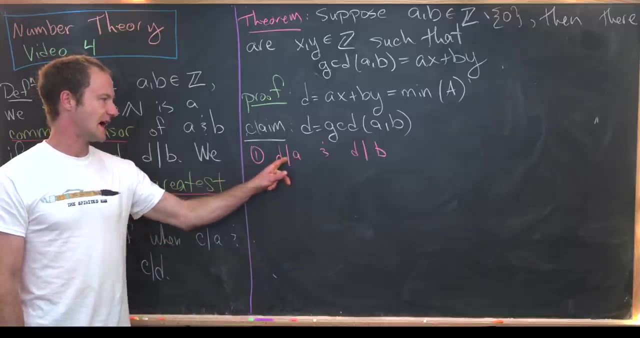 GCD of a and b. So we'll start by proving that it is a common divisor of a and b, In other words, d divides a and d divides b. Okay, so let's maybe see how we can do that. Well, let's first start by dividing a by d. 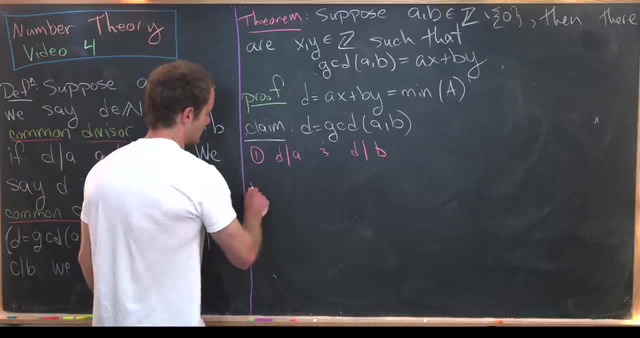 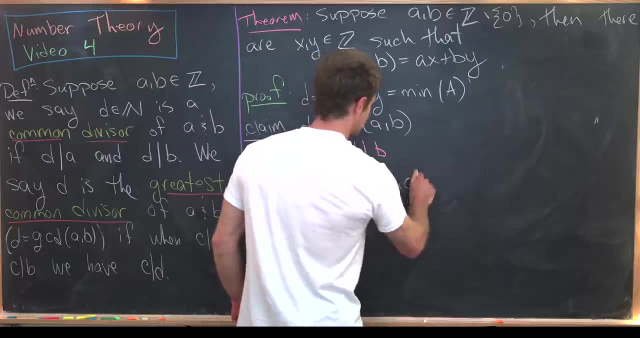 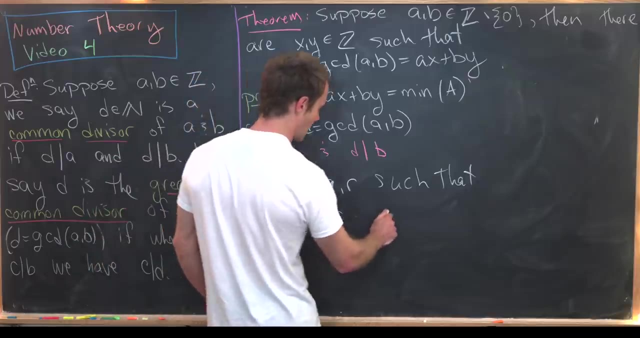 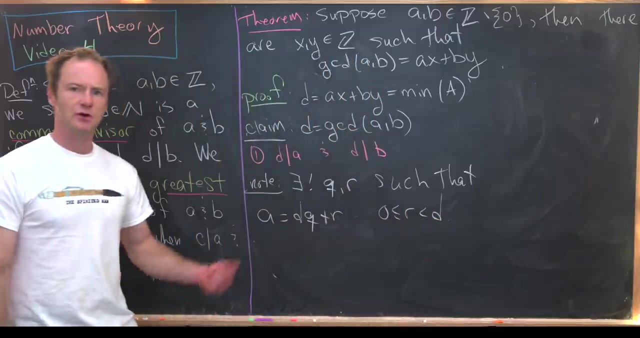 with remainder using the division algorithm. So let's notice that there exists unique q and r, Such that a equals d times q plus r, where 0 is less than or equal to r, which is strictly less than d. So again, that's just applying the division algorithm to d and a. Well, what can we do? 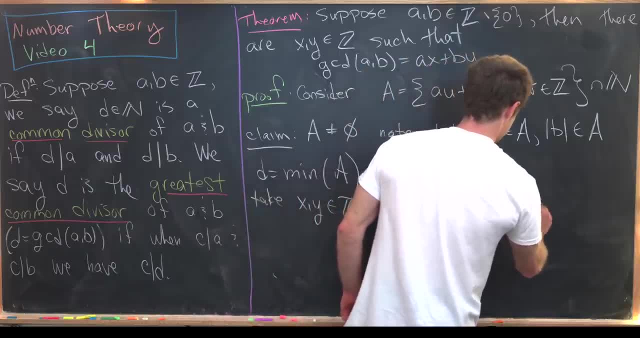 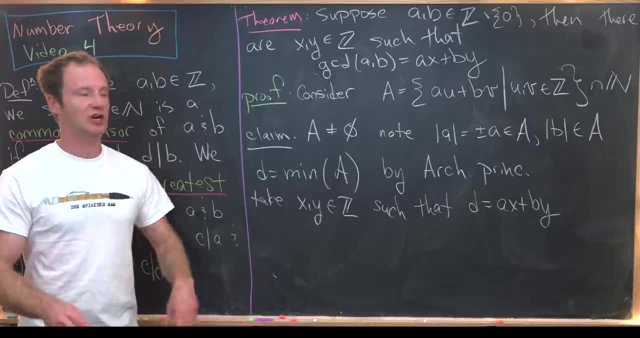 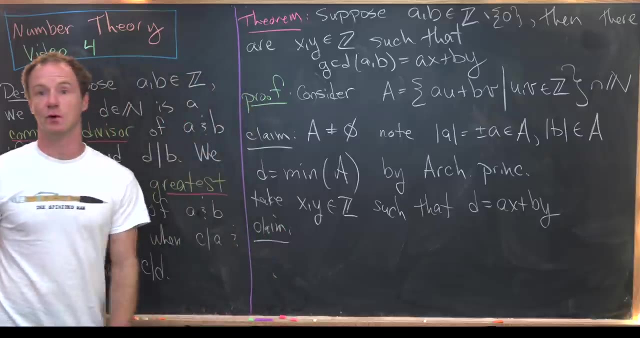 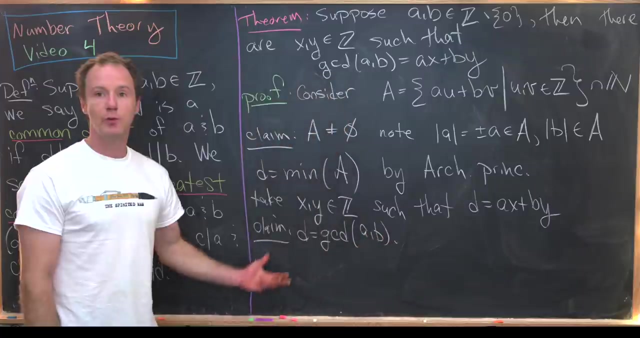 d equals ax plus by okay, but now look what we've got going on here. it looks like we're constructing exactly what we want, so that'll be our next claim is that we've actually constructed what we want. in other words, d is equal to the gcd of a and b, but we don't have room for that here, so 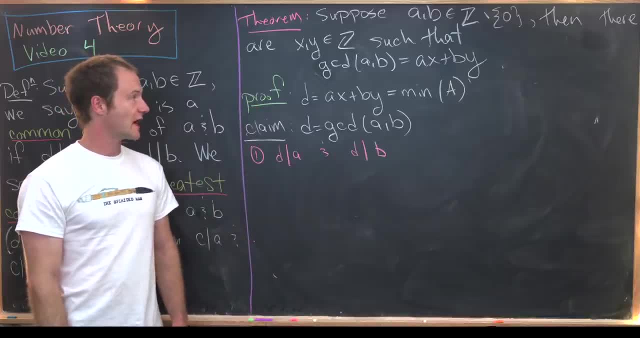 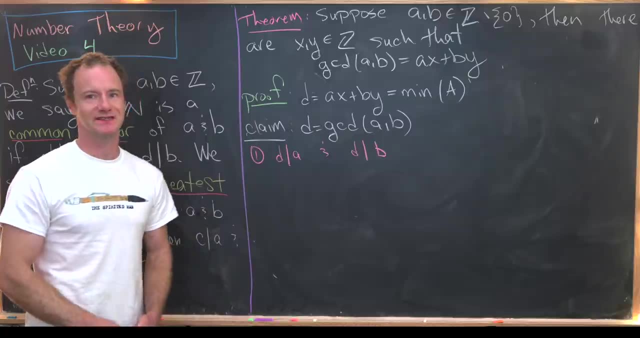 let's start over at the top. okay, so on the last board we constructed this number D as a linear combination of A and B as the minimum of some set A which we had on the last board. Now I want to claim that D is the GCD of A and 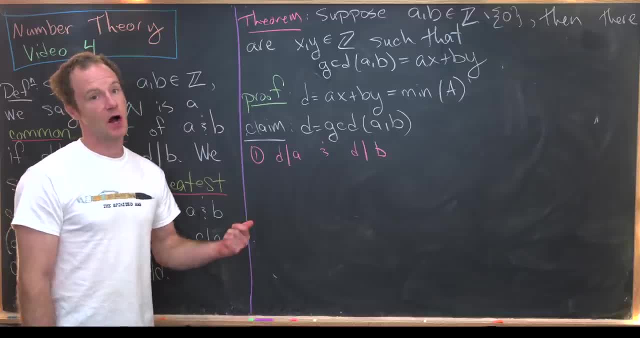 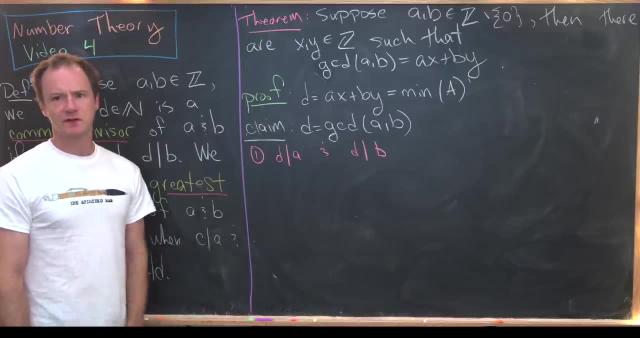 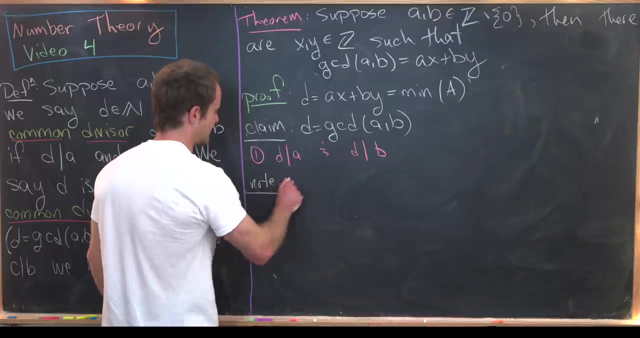 B. So we'll start by proving that it is a common divisor of A and B. In other words, D divides A and D divides B. Okay, so let's maybe see how we can do that. Well, let's first start by dividing A by D, with remainder using the division algorithm. So let's notice. 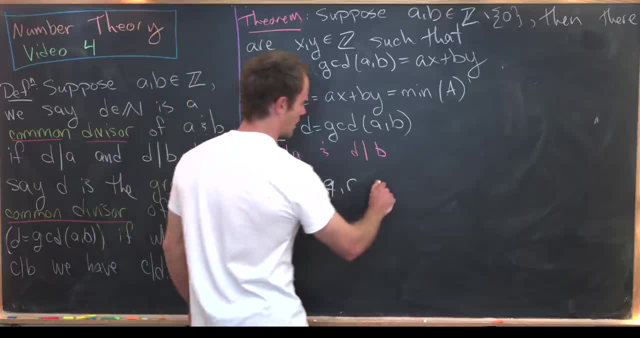 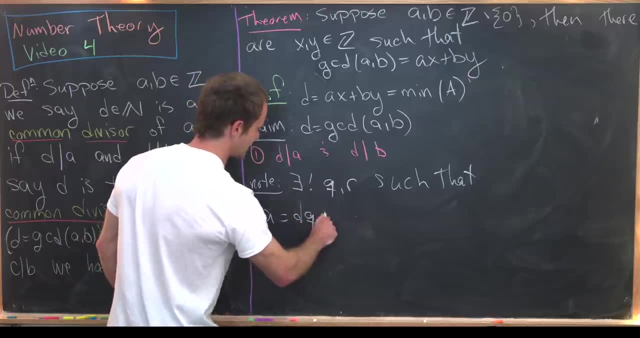 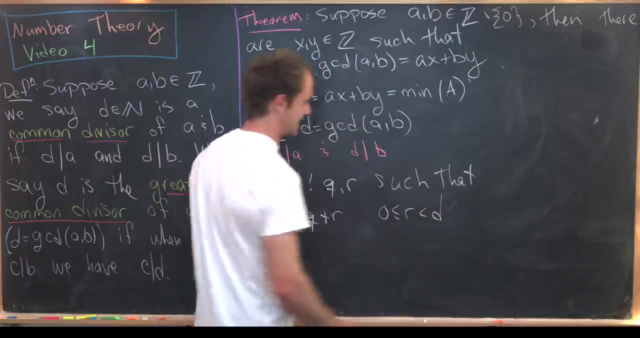 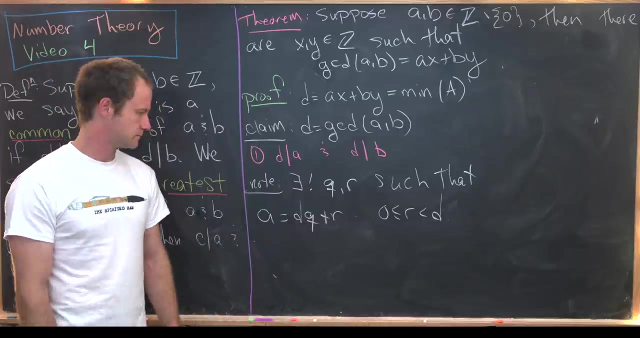 that there exists unique Q and R, such that A equals D times Q plus R, where zero is less than or equal to R, which is strictly less than D. So again, that's just applying the division algorithm to D and A. Well, what can we do from there? 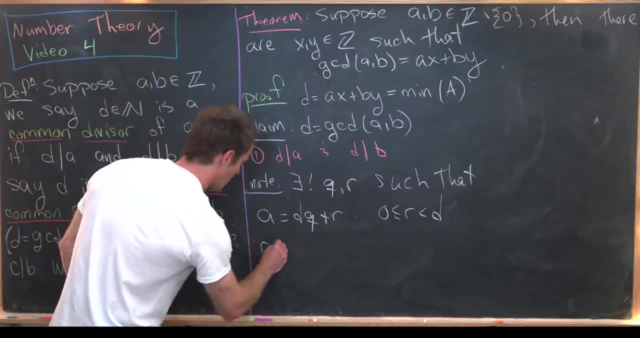 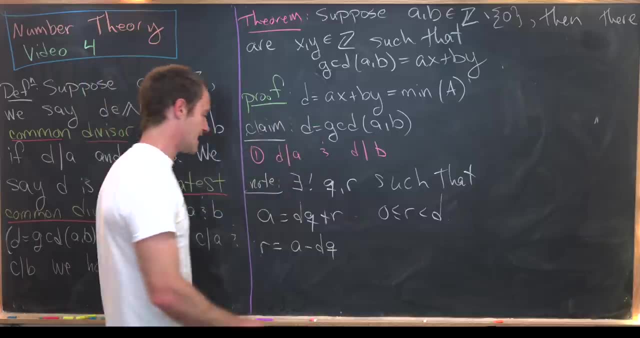 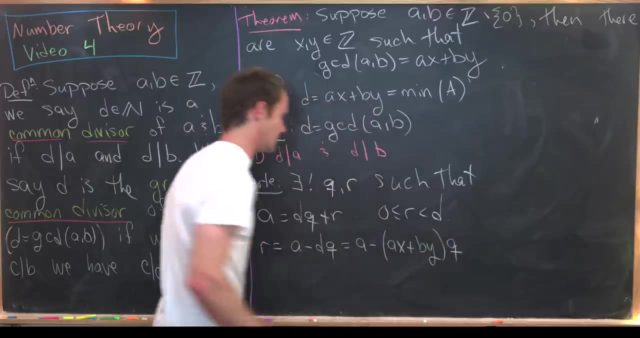 Well, I can solve this for R. So let's notice that R is equal to A minus D Q, But recall that D was equal to AX plus BY. so here we have A minus AX plus BY times Q, But now we can put this in terms of A and B. 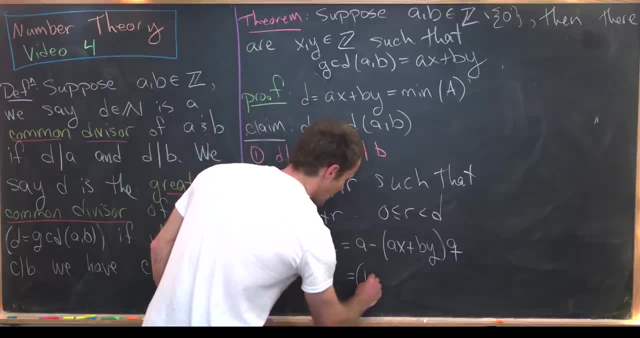 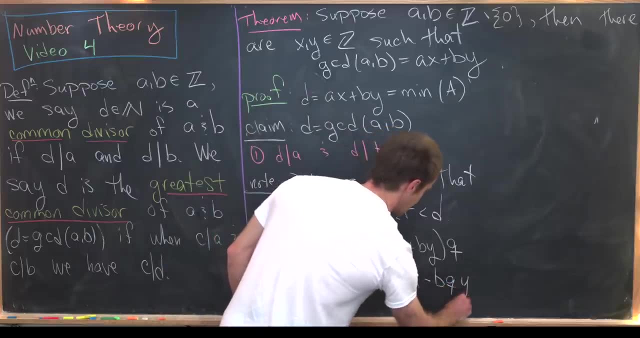 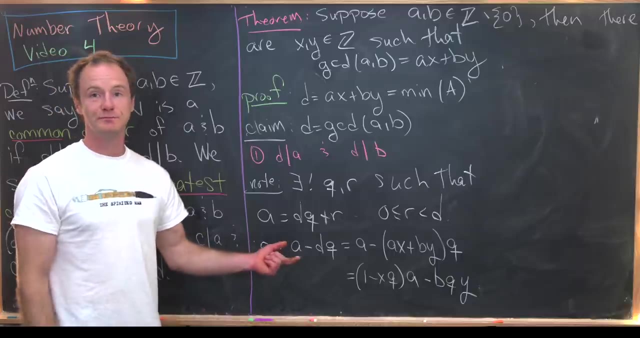 In other words, like rearrange this notice: we have 1 minus x times q times a, minus b times q times y. Well, look, that's a linear combination of a and b, which means it's either in the set a or it's equal to 0.. 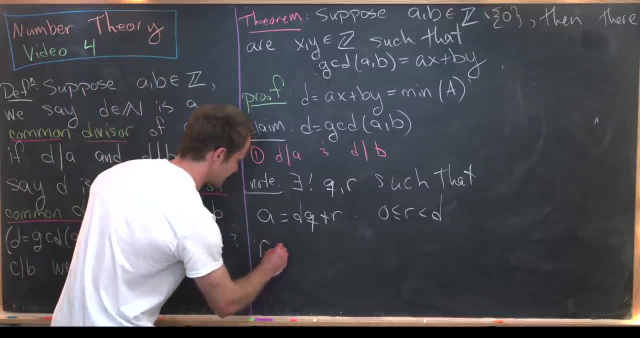 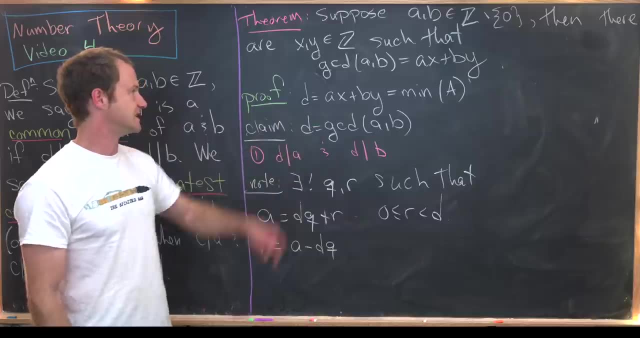 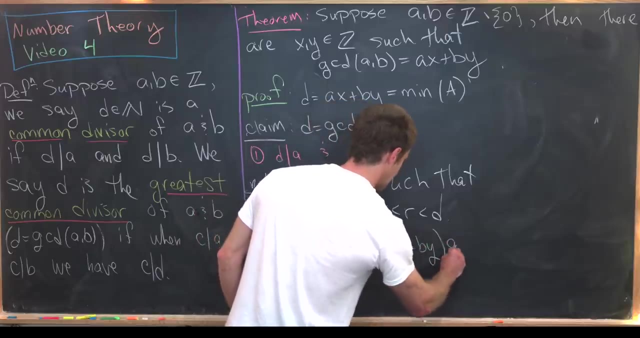 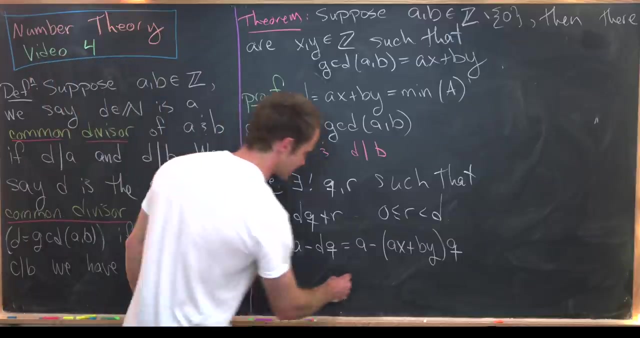 from there. Well, I can solve this for r. So let's notice that r is equal to a minus dq, But recall that d was equal to ax plus by. So here we have a minus ax plus by times q. Okay, but now we can put this in terms of a and b, In other words like rearrange this. 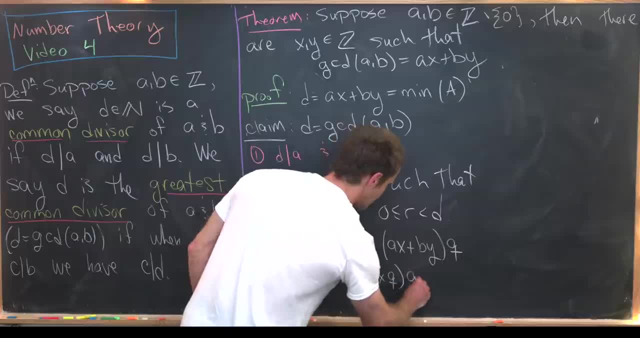 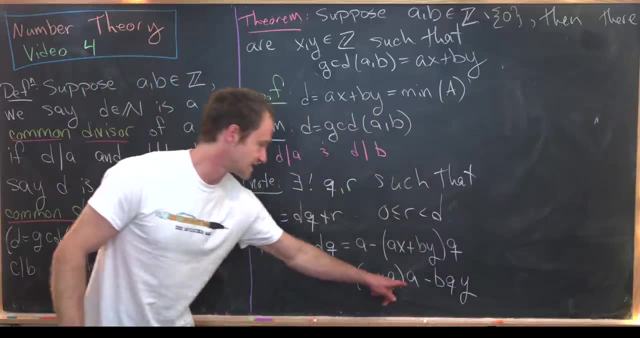 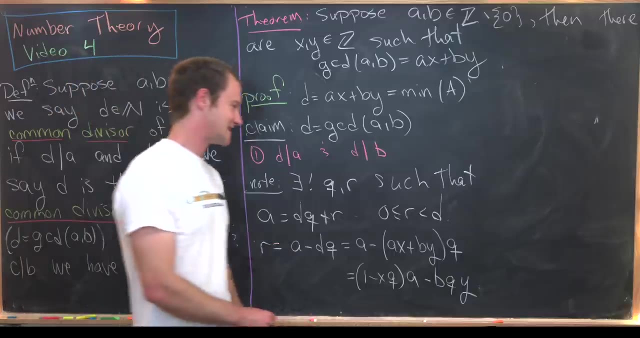 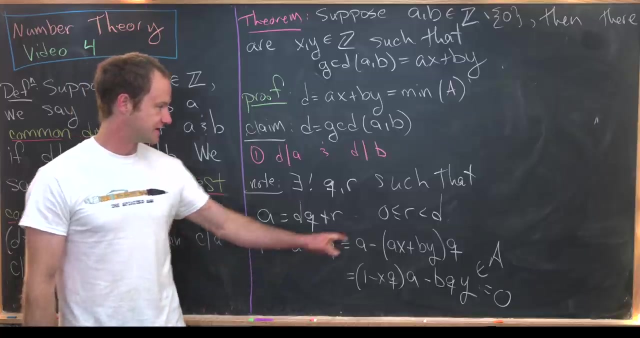 Notice we have 1 minus x times q times a, minus b times q times y. Well, look, that's a linear combination of a and b, which means it's either in the set a or it's equal to 0. Now, how do we know that? Well, look, r is between 0 and d, So that means it's. 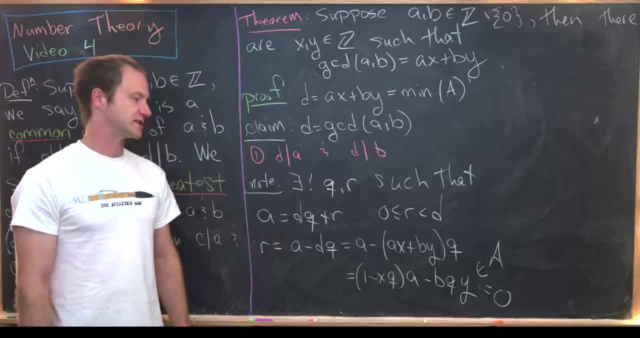 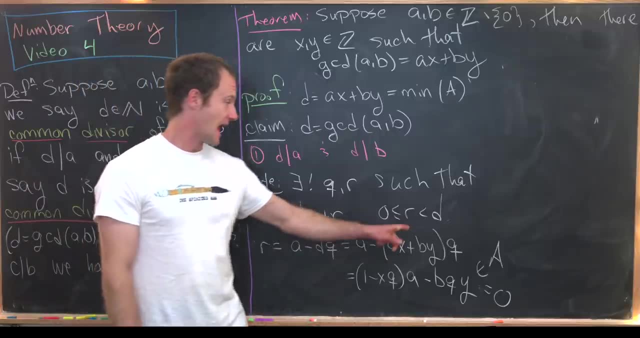 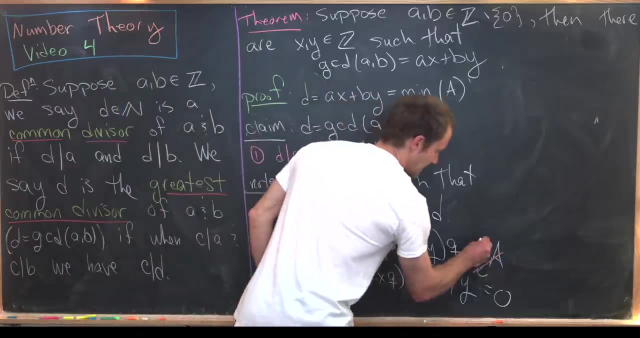 either a natural number already or it's equal to 0.. Notice, if it's a natural number, that means that it's in A. But if it's in A, it's less than the smallest element from A, So that's impossible. So it being in A is not a possibility which. 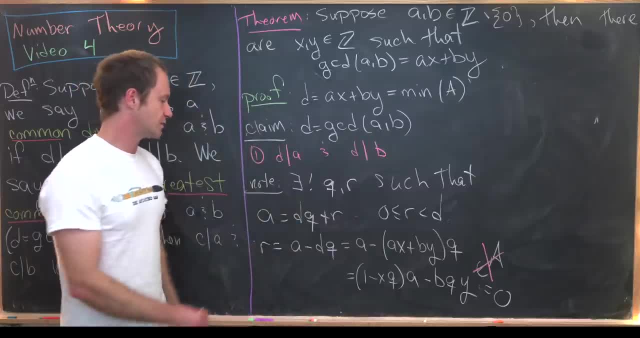 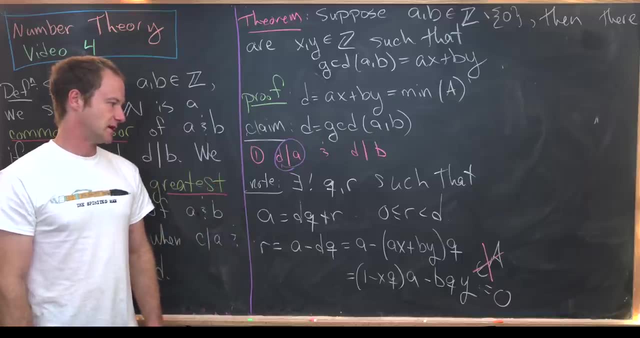 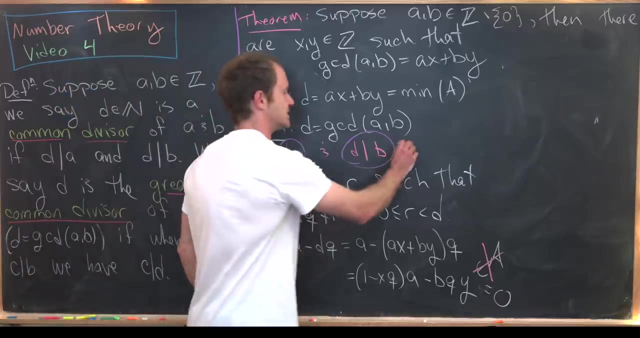 means it's equal to 0.. But if the remainder is equal to 0, that means we've proven that D divides A. And then very, very similarly, really, just switching A with B, we'll see that D also divides B. So that means: check, We've got that, it's. 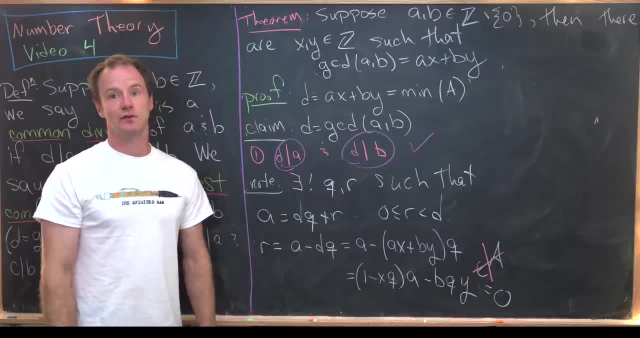 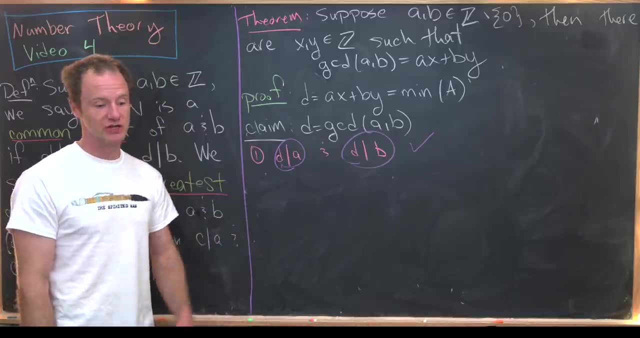 a common divisor. Now we just need to show that it is the greatest common divisor. Okay, like I said, we just got done proving that D was a common divisor of A and B. Now we want to show that it's a common divisor of A and B. Now we want to show that D is the greatest common divisor of A and B. Now we want to show that. 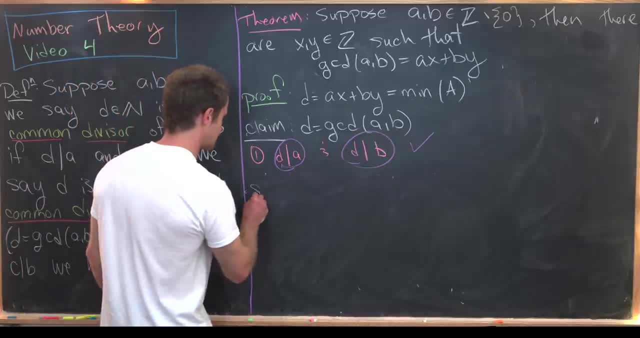 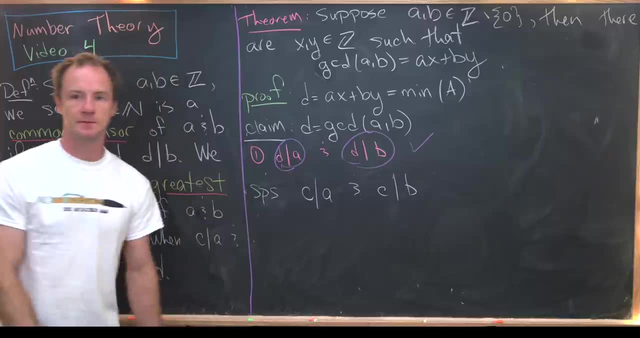 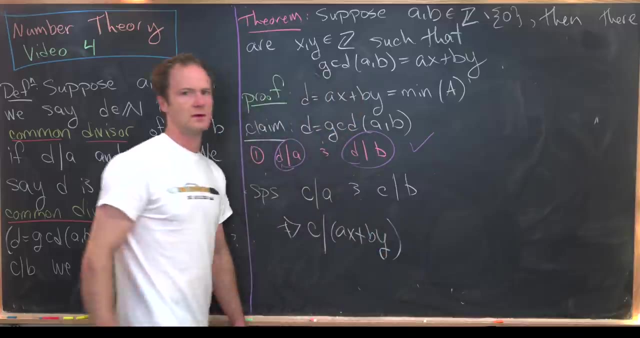 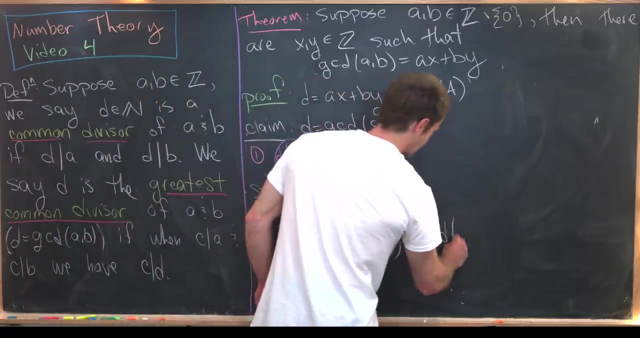 it's the greatest common divisor. So let's suppose that we have another common divisor, C, which divides A and it divides B. But notice that means that C divides AX plus BY by, something we proved in a previous video. But if C divides AX plus BY, that's exactly the same thing as saying: 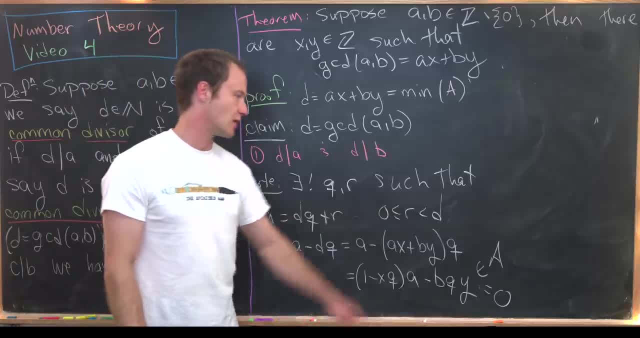 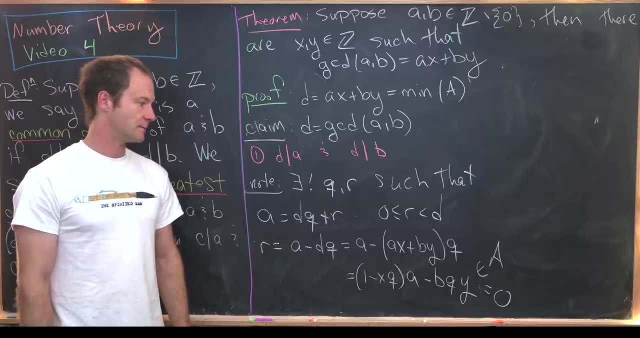 Now, how do we know that? Well, look, r is between 0 and d, So that means it's either a natural number already or it's equal to 0. Notice: if it's a natural number, that means that it's in a. 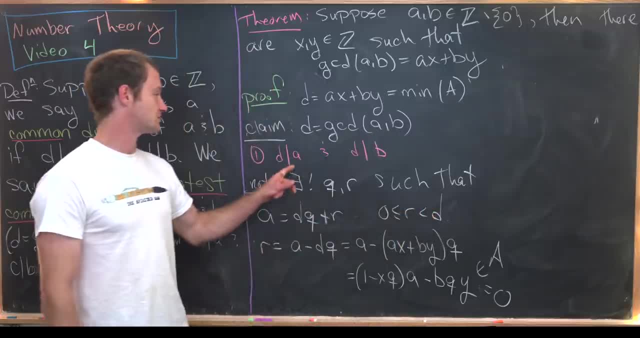 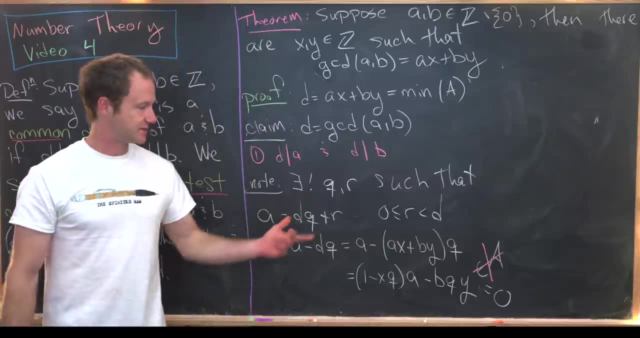 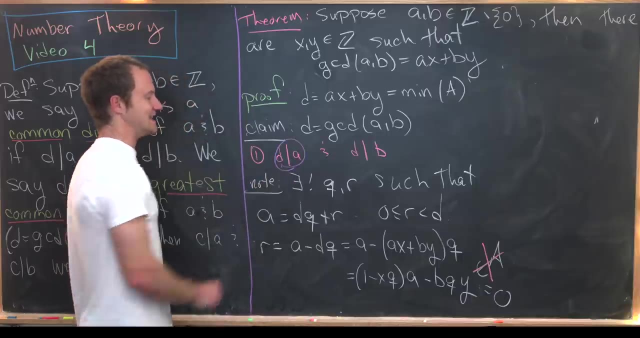 But if it's in a, it's less than the smallest element from a, So that's impossible. So it being in a is not a possibility, which means it's equal to 0.. But if the remainder is equal to 0, that means we've proven that d divides a. 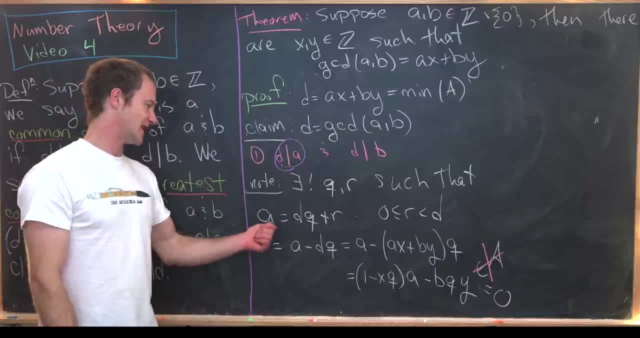 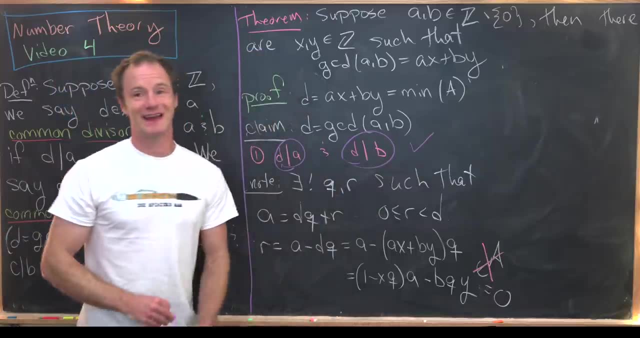 And then b And very, very similarly. really, just switching a with b, we'll see that d also divides b. So that means check, we've got that it's a common divisor. Now we just need to show that it is the greatest common divisor. 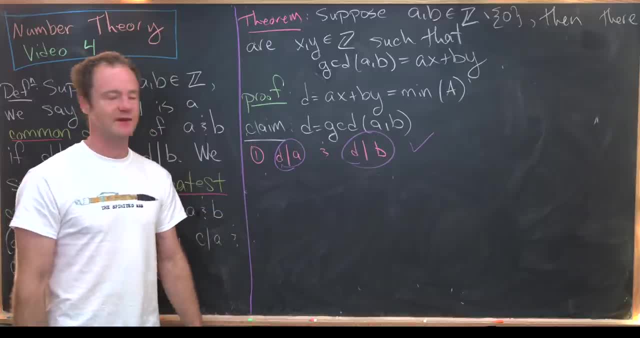 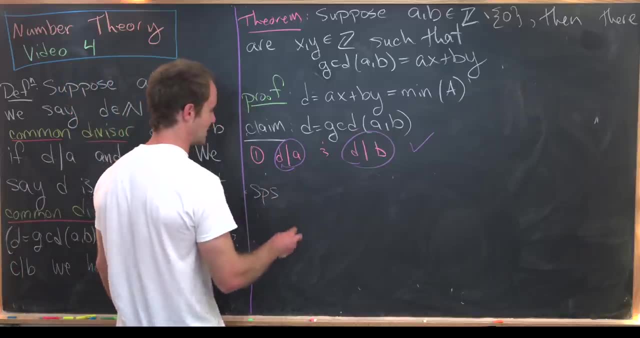 Okay, like I said, we just got done proving that d was a common divisor of a and b. Now we want to show that it's the greatest common divisor. So let's suppose that we have another common divisor, c, which divides a. 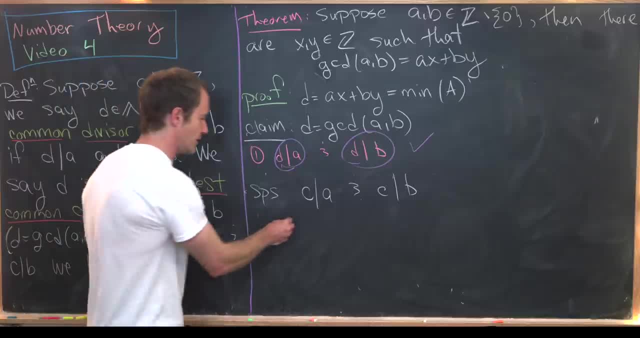 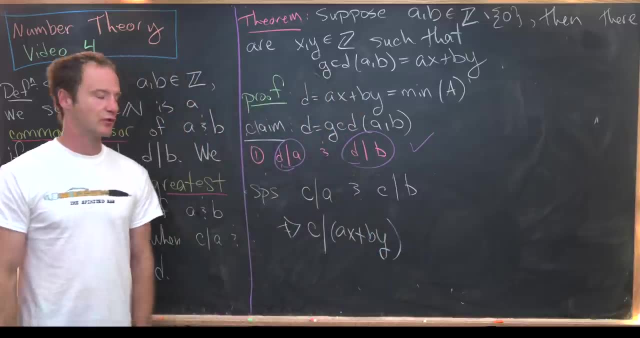 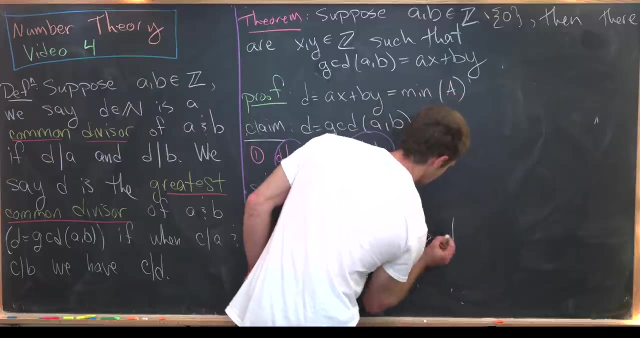 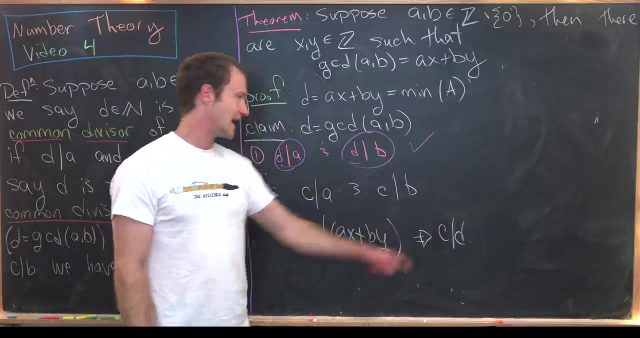 And it divides b. But notice that means that c divides ax plus by by, something we proved in a previous video. But if c divides ax plus by, that's exactly the same thing as saying that c divides d. So we started with a common divisor and we showed that it divided our would-be greatest common divisor. 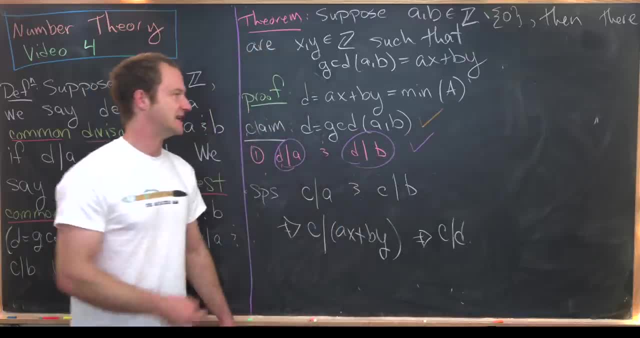 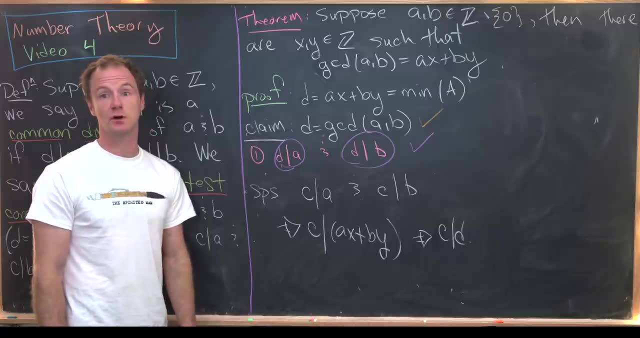 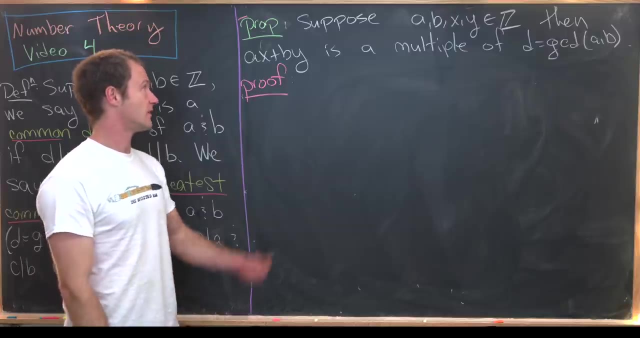 So that finishes. So that finishes this proof that d is the gcd of a and b, which is exactly what we wanted to show. Okay, so let's maybe get rid of this and we'll move on to some other ideas. So our next little result is a proposition involving objects of the form ax, plus by: 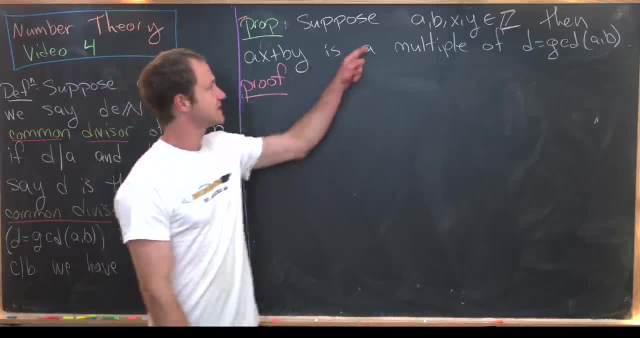 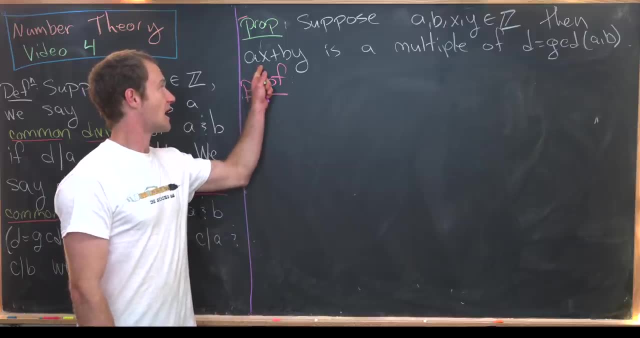 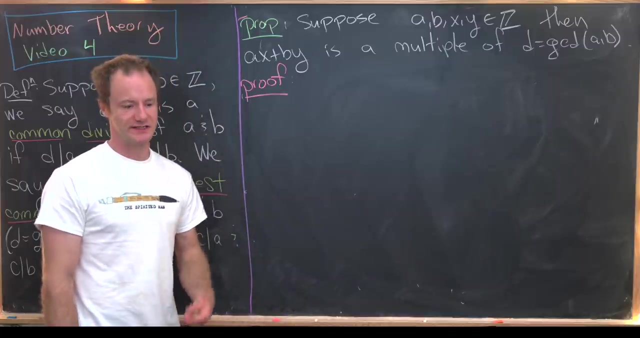 and how they're related to the gcd. So let's suppose that a, b, x and y are all integers, Then This object, ax plus by, is always a multiple of the gcd of a and b, which I'll call d. 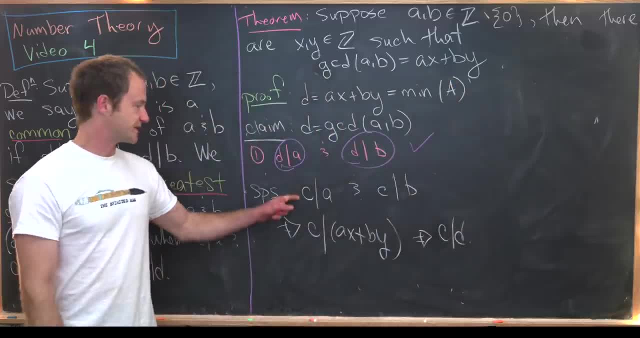 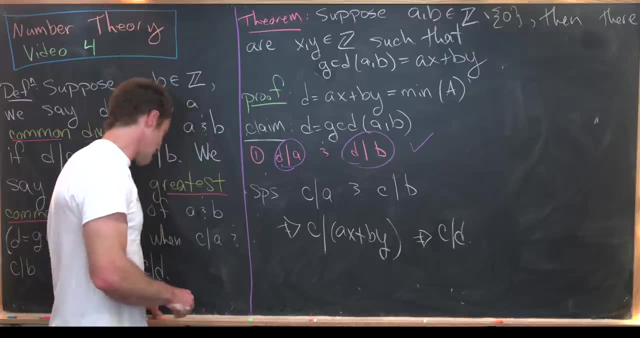 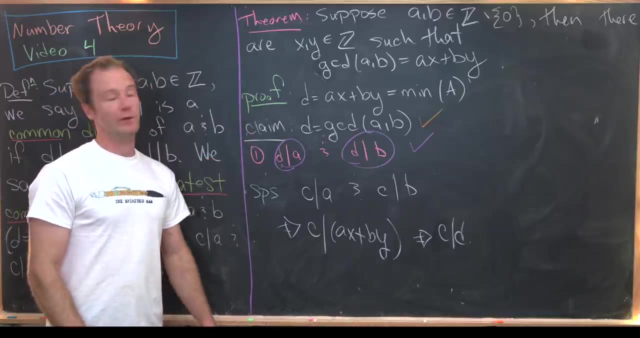 that C divides D. So we started with a common divisor and we showed that it divided our would be greatest common divisor. So that finishes this proof that D is the GCD of A and B, which is exactly what we wanted to show. Okay, so let's maybe get rid of this and we'll move on to some other. 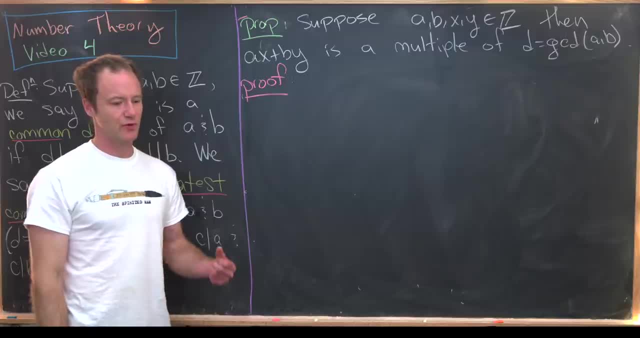 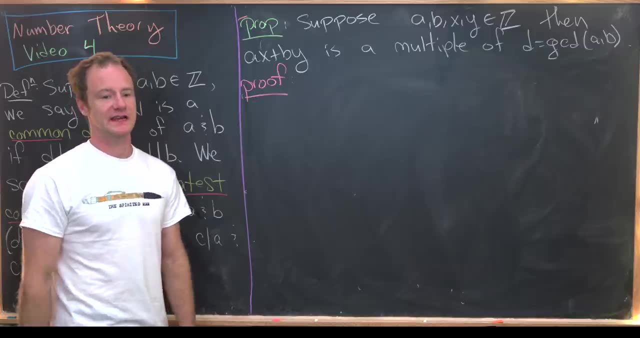 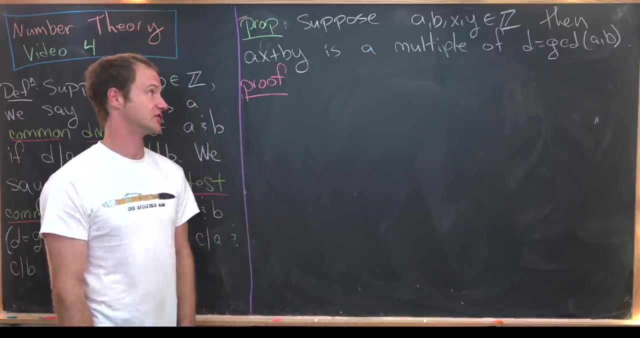 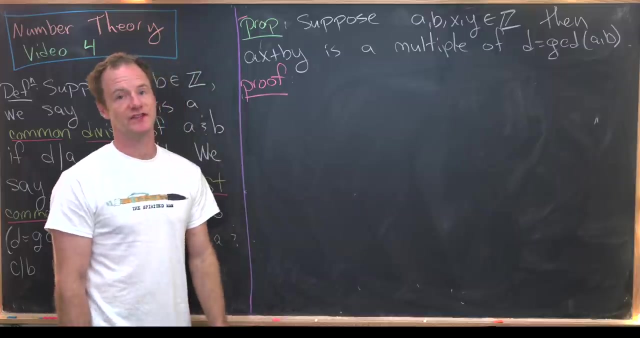 ideas. So our next little result is a proposition involving objects of the form AX plus BY And how they're related to the GCD. So let's suppose that A, B, X and Y are all integers, Then this object, AX plus BY, is always a multiple of the GCD of A and B, which I'll call D. So we 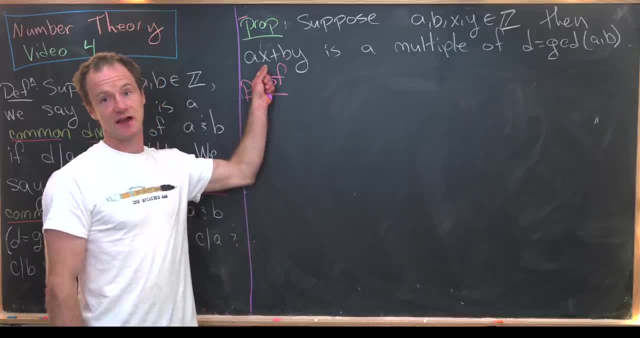 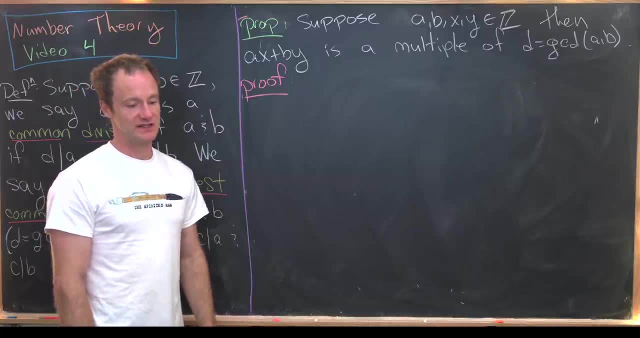 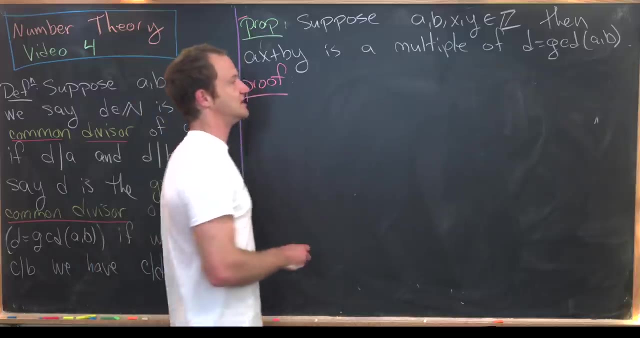 know that we can write the GCD in this form. Well, it turns out the only numbers that we can write in this form are multiples of the GCD of A and B of that GCD. Okay, so let's maybe see how this proof goes. Well, notice if D is the GCD of A. 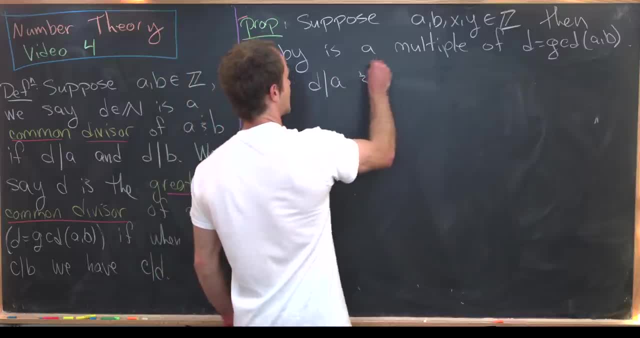 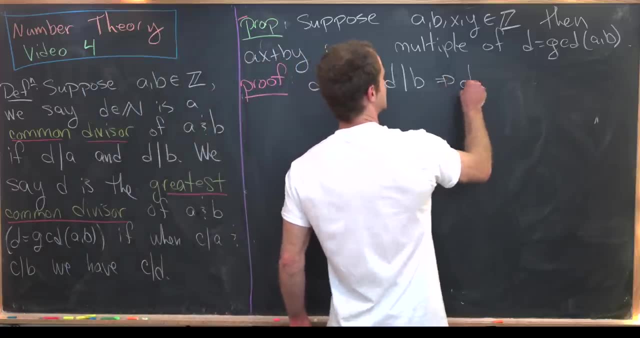 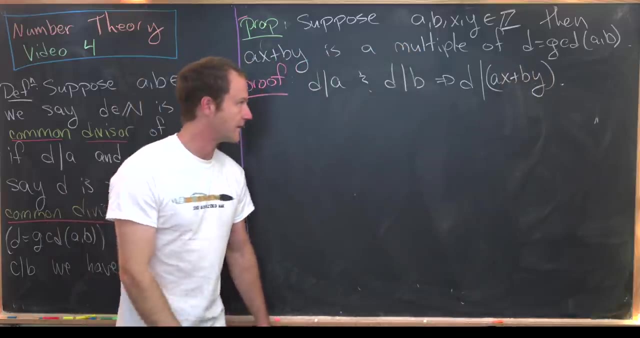 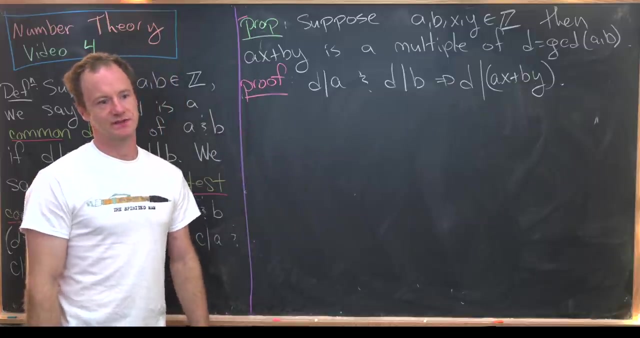 and B, then that means D divides A and D divides B. But if D divides A and D divides B, that means that D divides AX plus BY. That's going to be true for all X and Y. But saying that D divides that AX plus BY is the same thing as saying that AX plus BY is a multiple of D. Those are two. 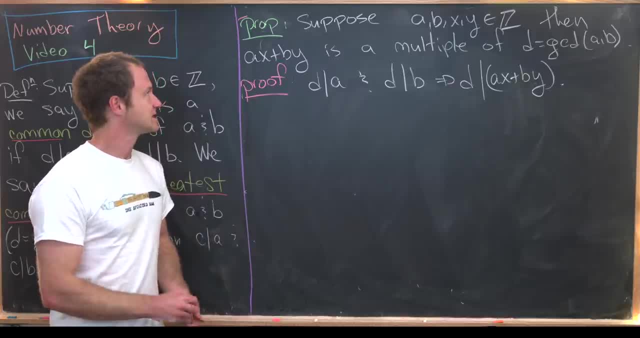 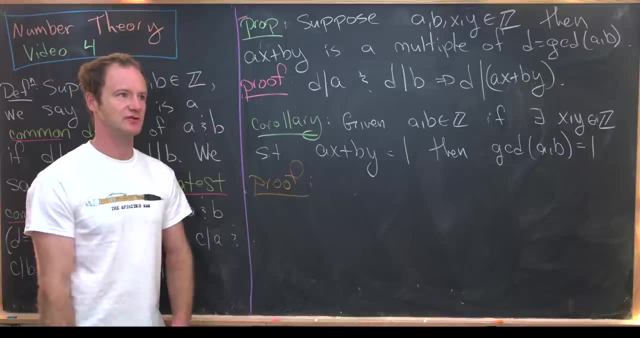 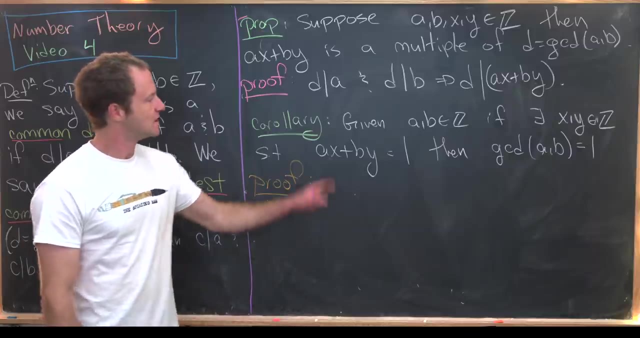 different ways of saying the same thing. Okay, so now let's look at a corollary of this proposition. So here's a super important corollary of this proposition which actually allows you to find out when things have a GCD of 1, when it might be tricky to do otherwise. So let's say we've got. integers A and B and there exists a corollary of this proposition. So let's say we've got integers A and B and there exists a corollary of this proposition. So let's say we've got integers A and B and there exists. 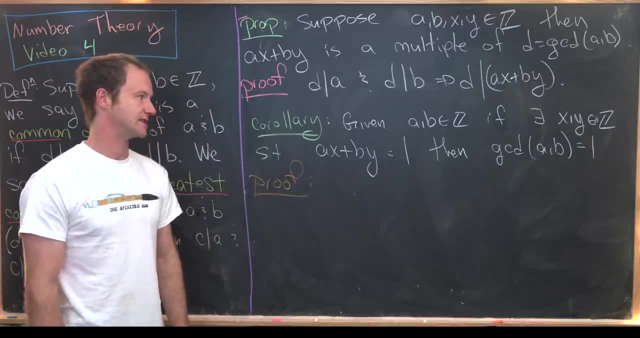 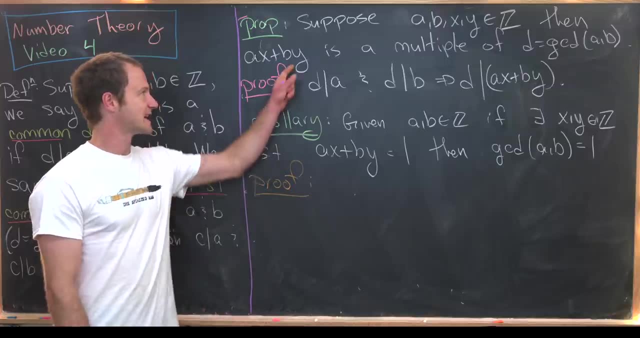 other integers, X and Y, such that AX plus BY is equal to 1.. Then the GCD of A and B is equal to 1.. So that's actually going to follow from this very, very quickly and it's pretty easy to show. 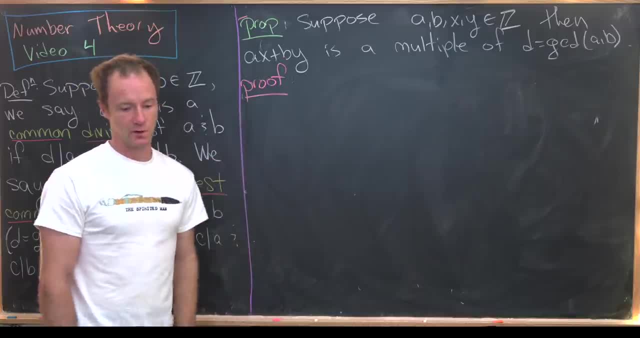 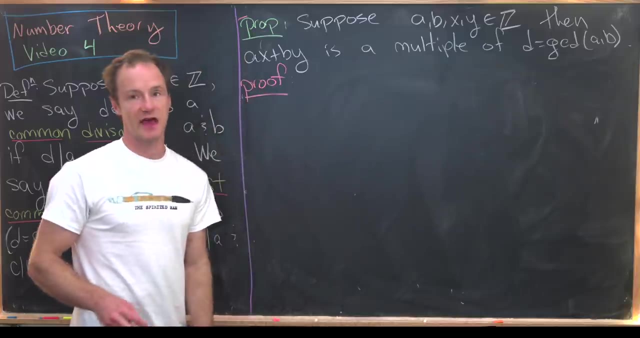 So we know that we can write the gcd in this form. Well, it turns out the only numbers that we can write in this form are multiples of that gcd. Okay, so let's maybe see how this proof goes. Well notice: if d is the gcd of a and b, then that means 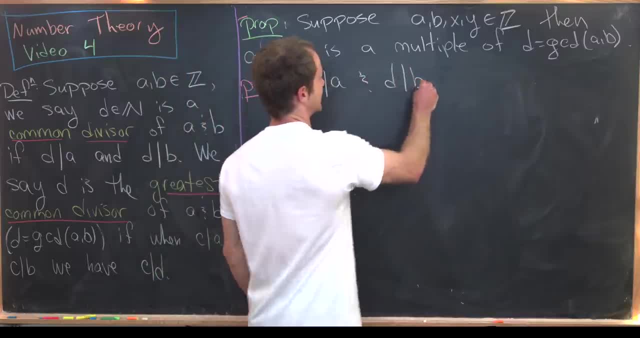 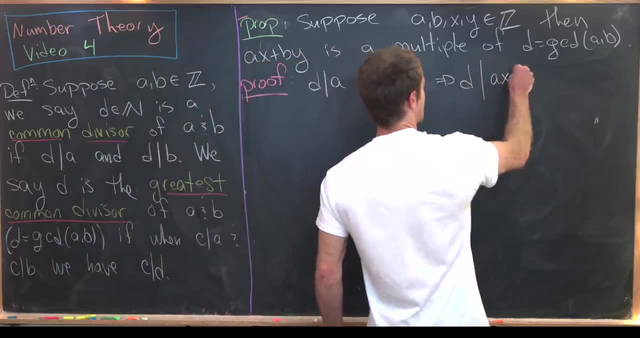 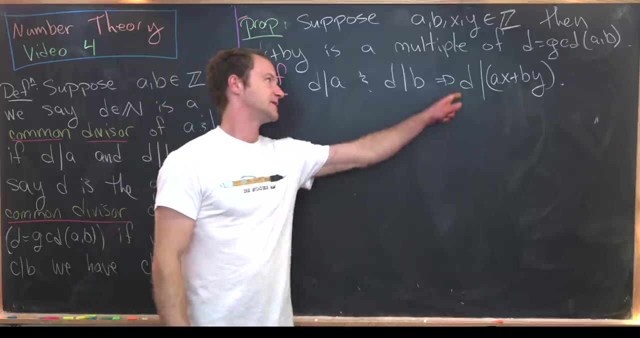 D divides a and b. D divides a and d divides b. But if d divides a and d divides b, that means that d divides ax plus by. That's going to be true for all x and y. But saying that d divides that ax plus by is the same thing as saying that ax plus by. 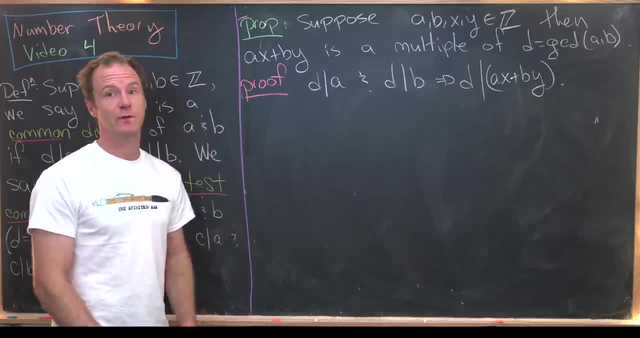 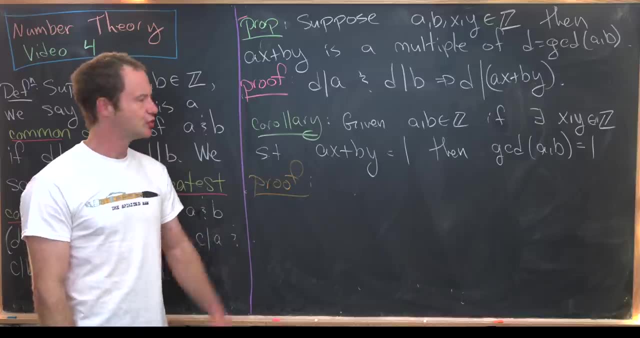 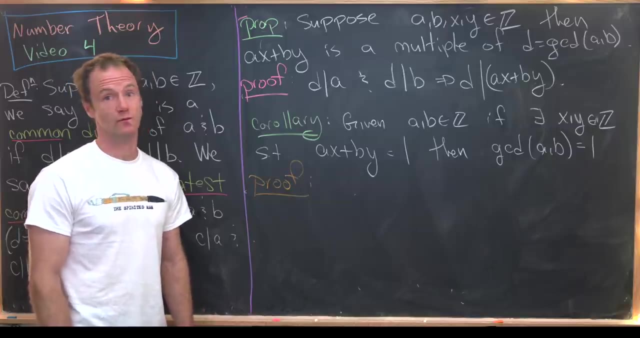 is a multiple of d. Those are two different ways of saying the same thing. Okay, So let's look at a corollary of this proposition. So here's a super important corollary of this proposition which actually allows you to find out when things have a gcd of 1, when it might be tricky to do otherwise. 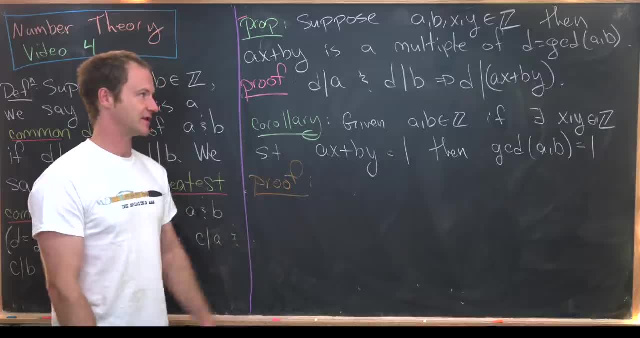 So let's say we've got integers a and b and there exist other integers, x and y, such that ax plus by is equal to 1.. Then the gcd of a and b is equal to 1.. So that's actually going to follow from this very, very simple proof. 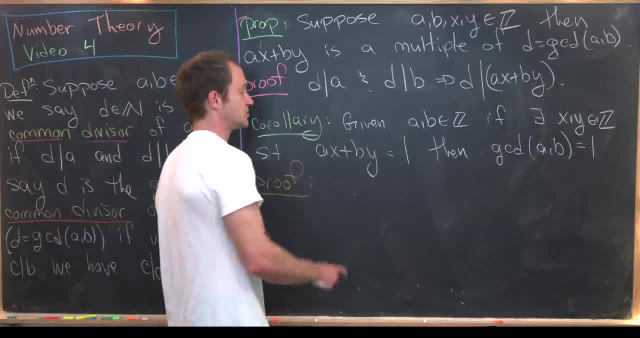 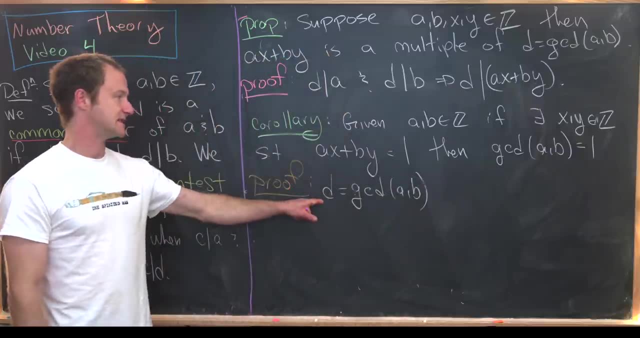 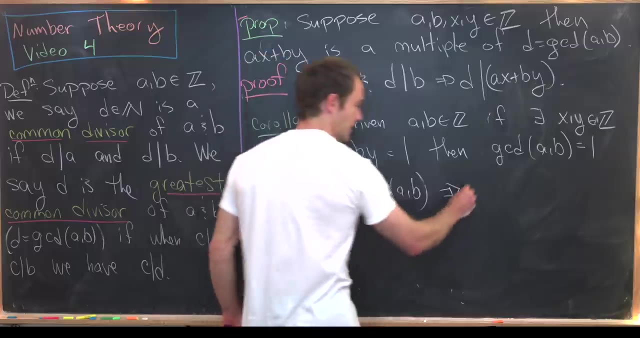 And it's pretty easy to show. So let's say that d is equal to the gcd of a and b, But that means that d divides ax plus by by this proposition. But ax plus by is 1.. So that means d divides 1.. 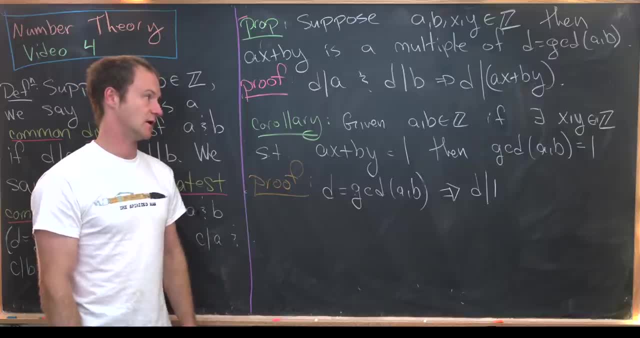 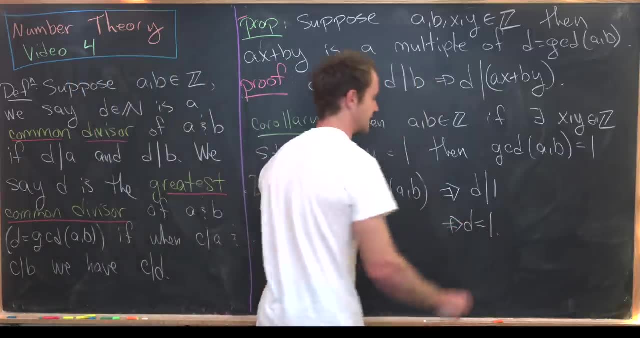 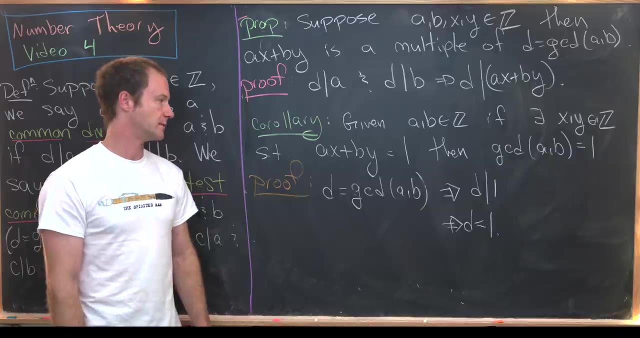 But there are only two integers that divide 1, plus and minus 1.. But gcds are always positive, So that means plus 1 is the only possibility for d. So here we've got: d is equal to 1.. In other words, the gcd of a and b are 1.. 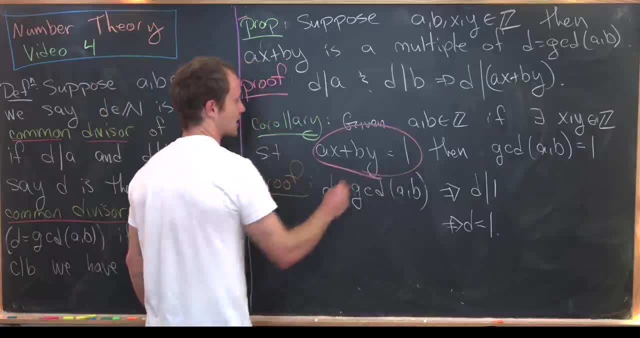 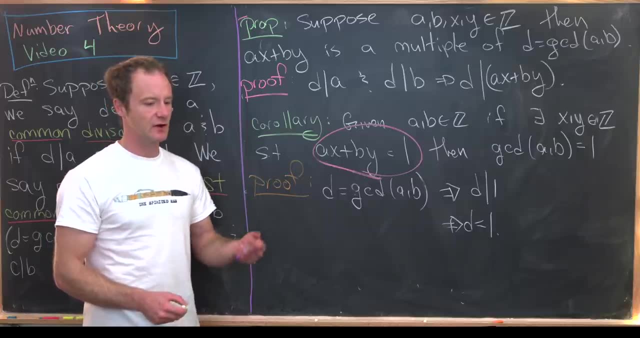 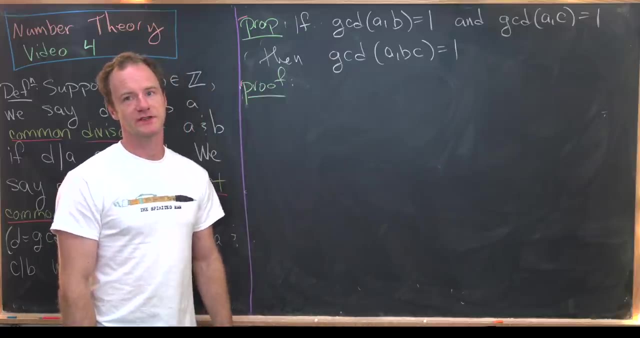 So if it is possible to take a linear combination of two integers and get 1, that means they are immediately relatively prime, Okay. So let's finish this video off with one proposition and one extension of this notion of greatest common divisor. So one more proposition. 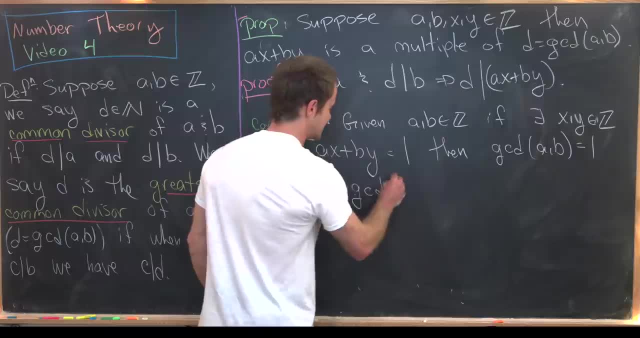 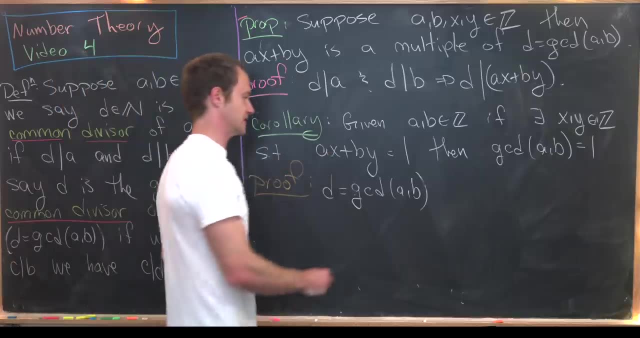 So let's say that D is equal to the GCD of A and B, But that means that D divides AX plus BY by this proposition, But AX plus BY is 1, so that means D divides AX plus BY by 1.. So that means: 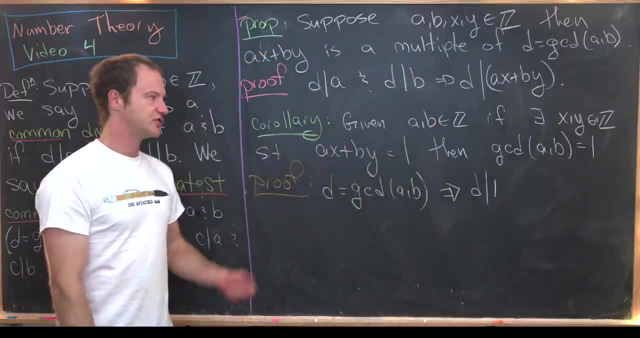 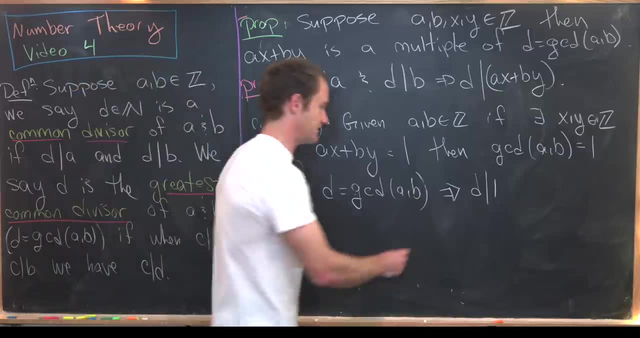 D divides 1, but there are only two integers that divide 1, plus and minus 1.. But GCDs are always positive, so that means plus 1 is the only possibility for D. So here we've got: D is equal. 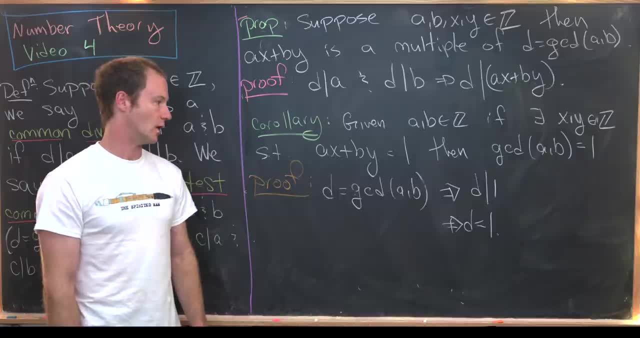 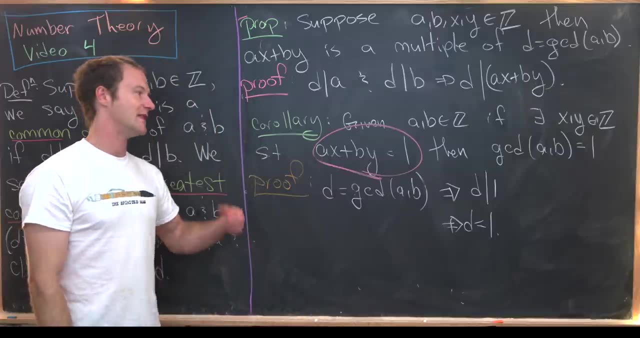 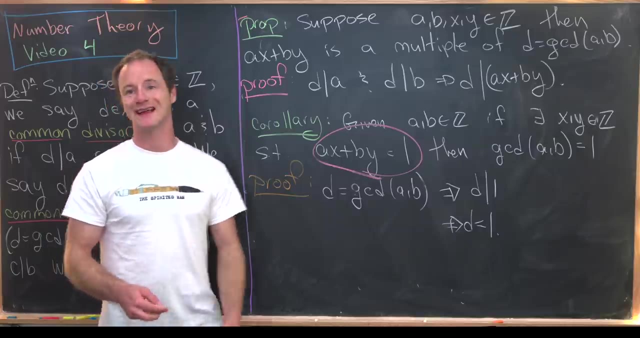 to 1.. In other words, the GCD of A and B are 1.. So if it is possible to take a linear combination of two integers and get 1, that means they are immediately relatively prime Okay. so let's finish this video off with one proposition and one extension of this notion. 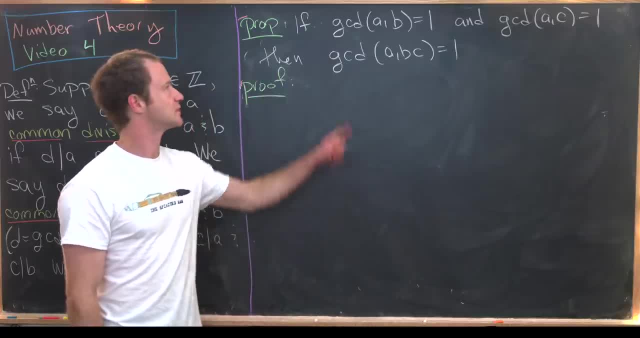 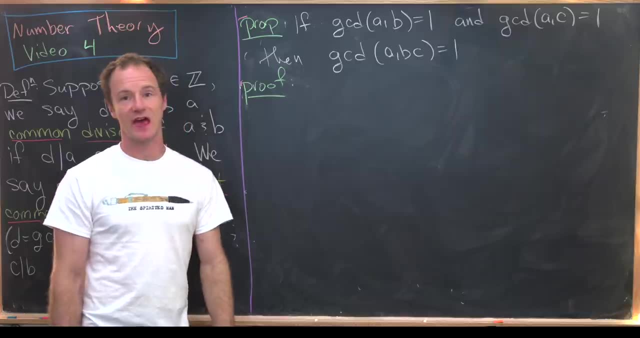 of greatest common divisor. So one more proposition. So if the GCD of A and B is 1, and the GCD of A and C is 1,, then the GCD of A and B times C is also 1.. So how can we do this? 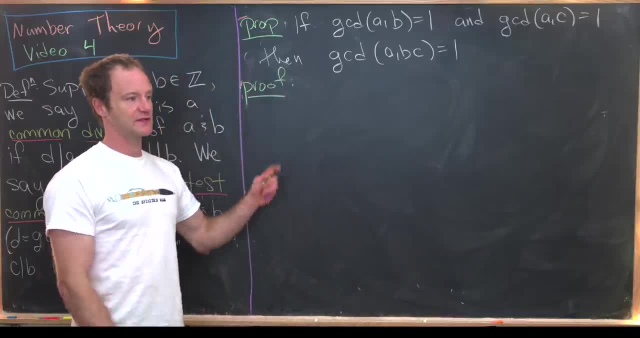 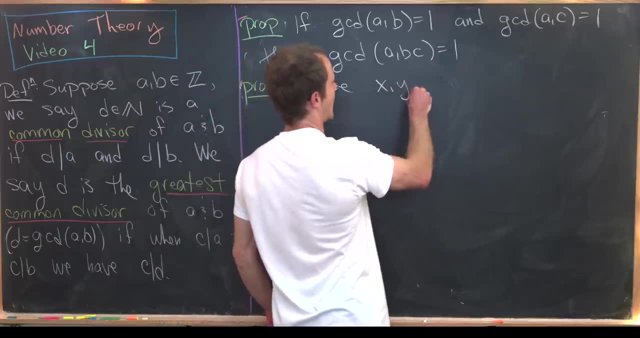 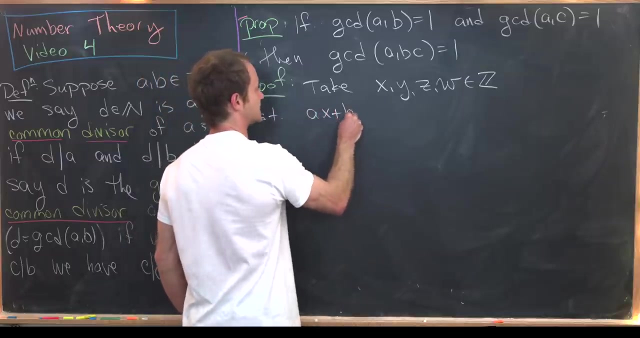 Well, we'll use the theorem that we had before, as well as the proposition and corollary that we just went over. So let's maybe go ahead and take X, Y, Z and W, which are all integers, such that AX plus BY is equal to the GCD of A and B. 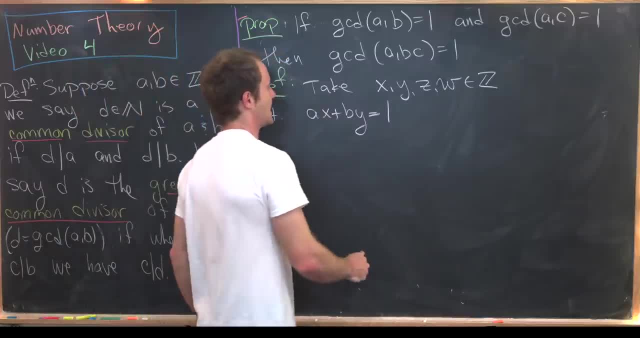 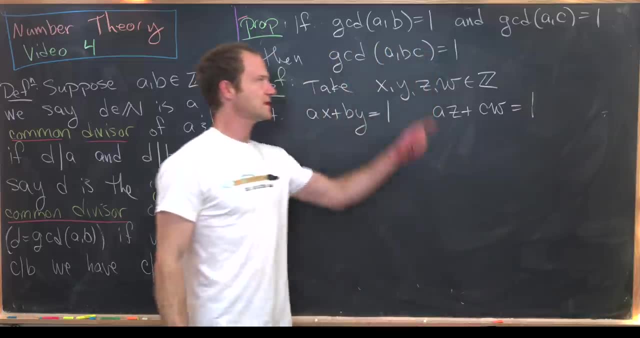 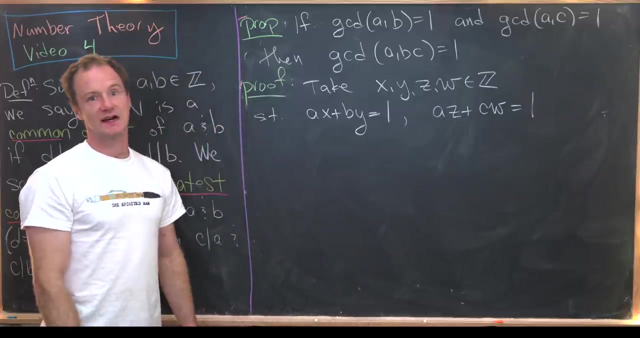 which is 1.. So that's possible by that theorem. And then AZ plus CW is equal to 1.. That's because the GCD of A and C is 1, again by that theorem. Now we'll just multiply both sides of this. 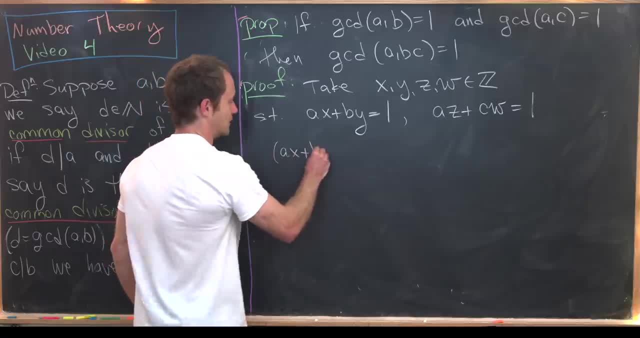 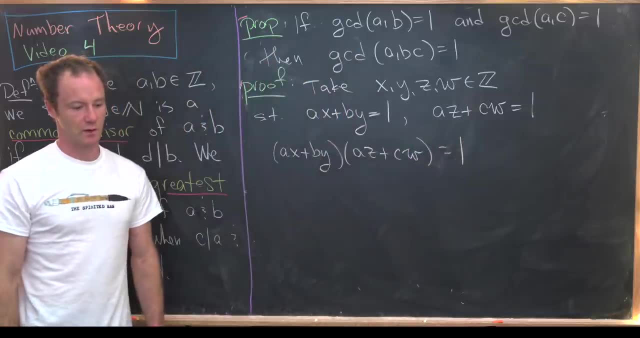 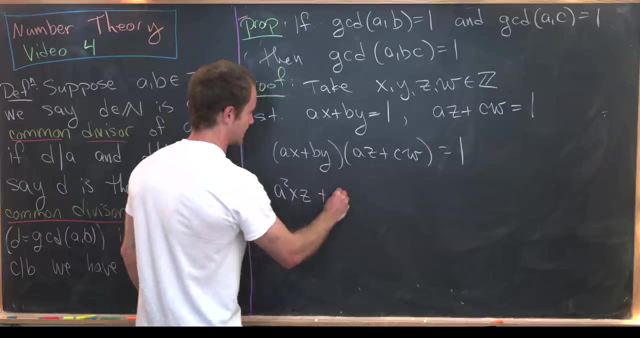 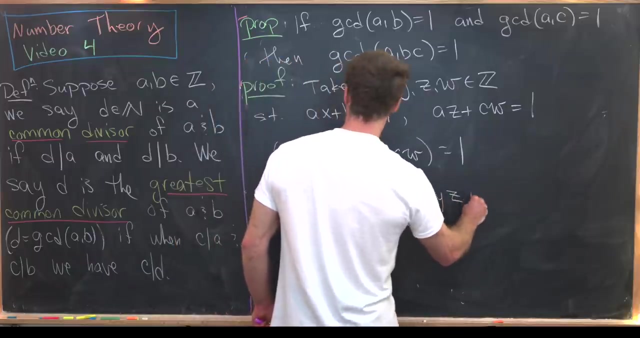 equation. So that tells us that AX plus BY times AZ plus CW is equal to 1 times 1, which is equal to 1.. But now let's multiply that out. So here we'll get A squared: XZ plus AC, XW plus AB times YZ plus. 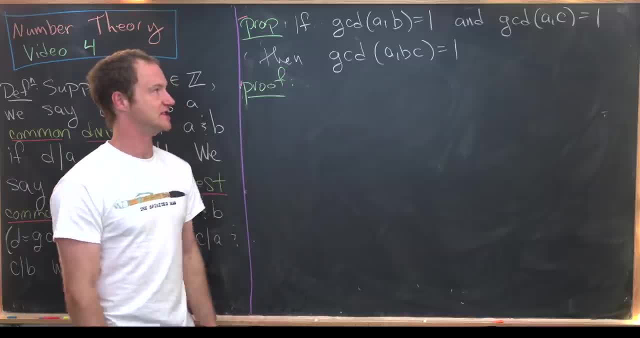 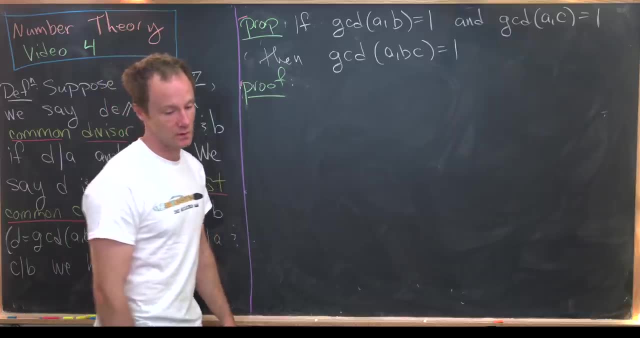 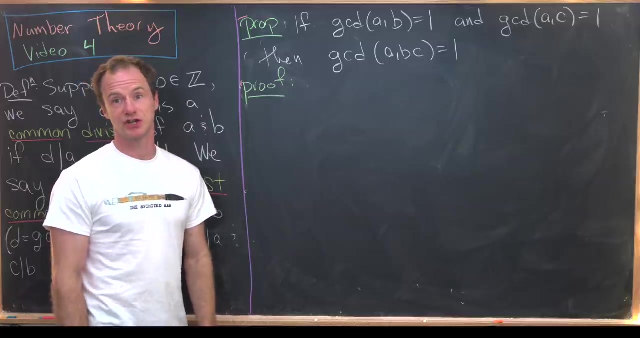 So if the gcd of a and b are 1.. And the gcd of a and c is 1. Then the gcd of a and b times c is also 1.. So how can we do this? Well, we'll use the theorem that we had before, as well as the proposition and corollary that 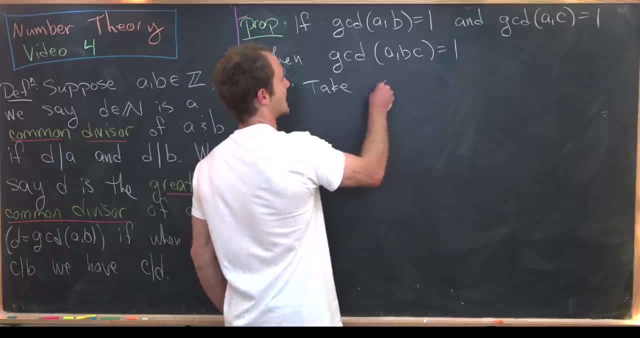 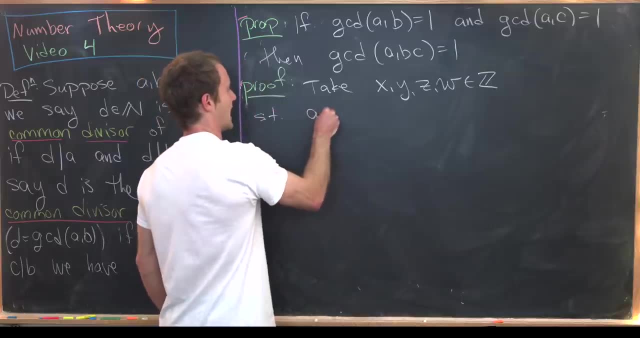 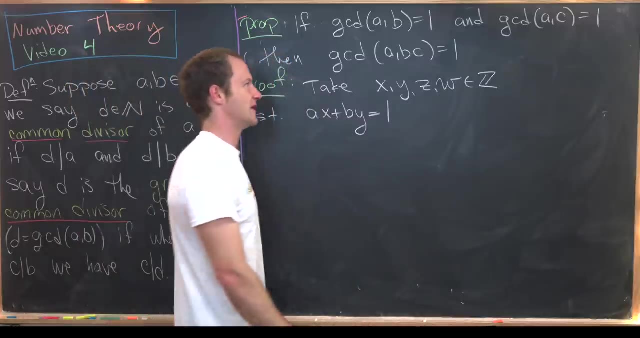 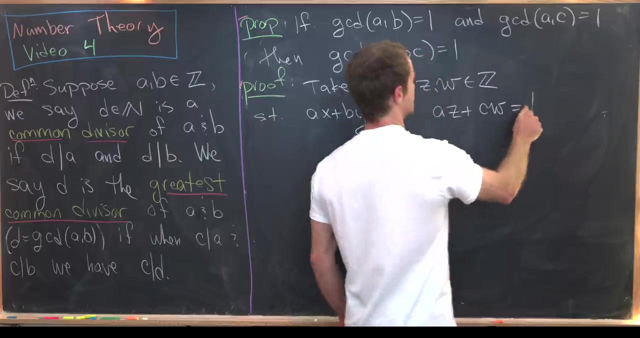 we just went over. So let's maybe go ahead and take x, y, z and w, which are all integers such that ax plus by is equal to 1. So that's possible by that theorem, And then az plus cw is equal to 1.. 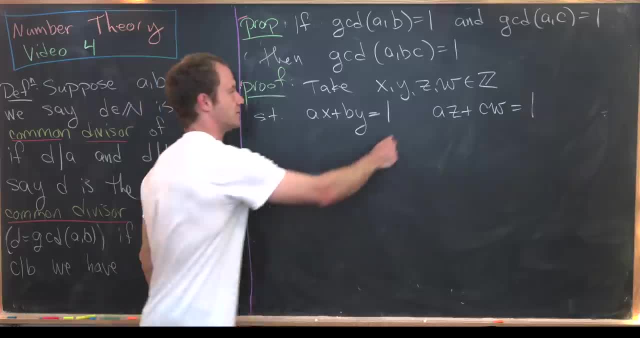 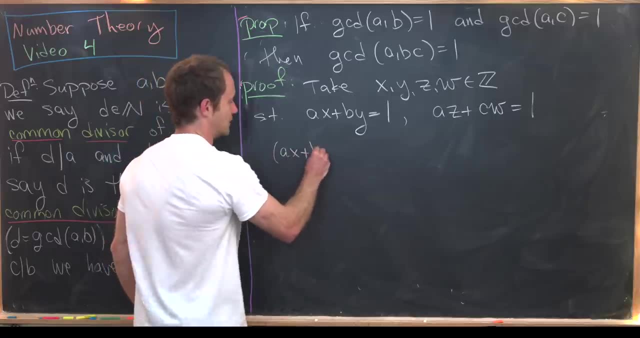 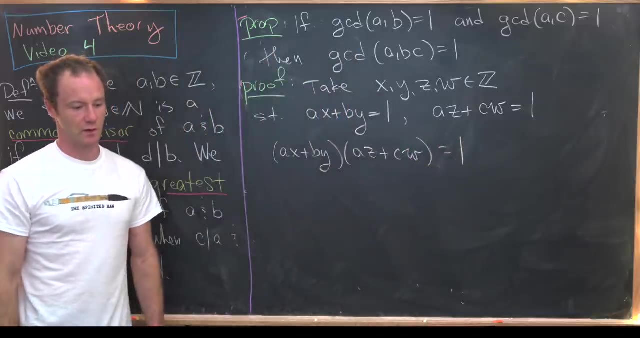 That's because the gcd of a and c is 1.. Again by that theorem. Now we'll just multiply both sides of this equation, So that tells us that ax plus by times az plus cw is equal to 1 times 1. Which is equal to 1.. 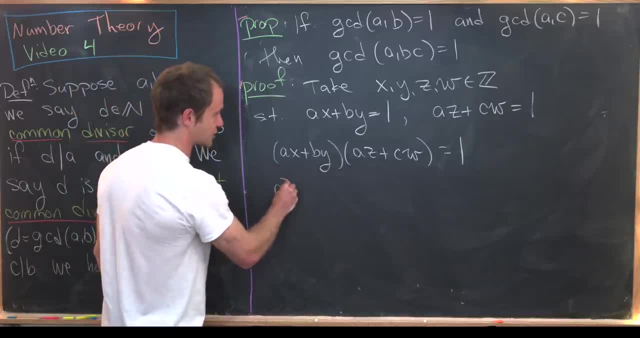 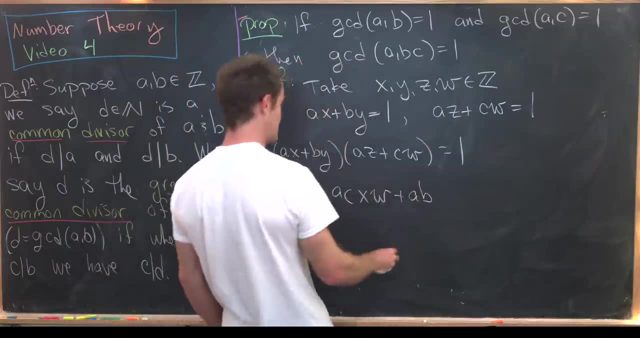 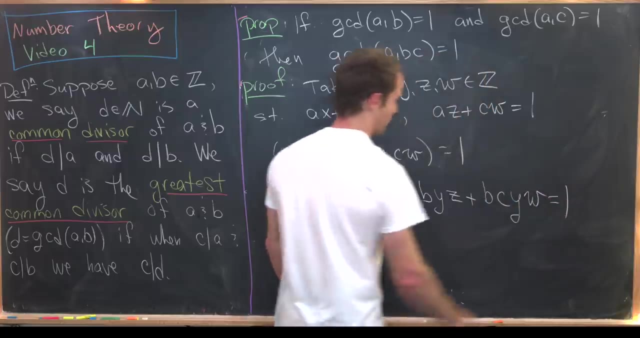 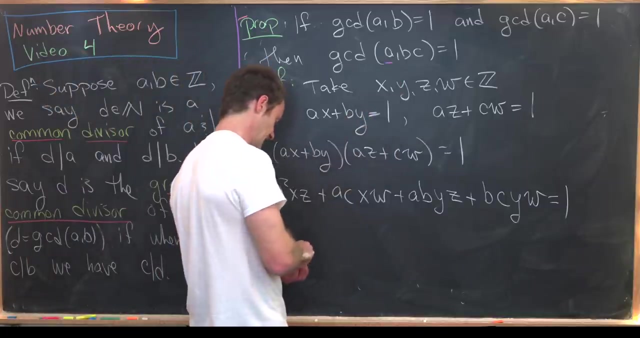 But now let's multiply that out. So here we'll get a squared xz plus ac, xw plus ab times, yz plus bc times, yw equals 1.. But now let's look at what our goal is. Our goal is to show that the gcd of a with bc is equal to 1.. 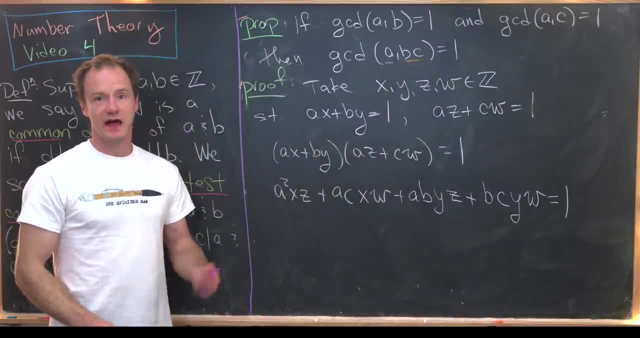 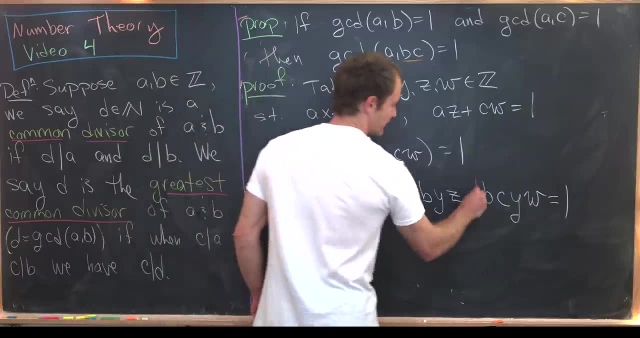 So let's look at what our goal is. Our goal is to show that the gcd of a with bc is equal to 1.. But we can do that if we can write a linear combination of a and bc is equal to 1.. We'll notice here we've got bc and then in all of the rest of these terms we have 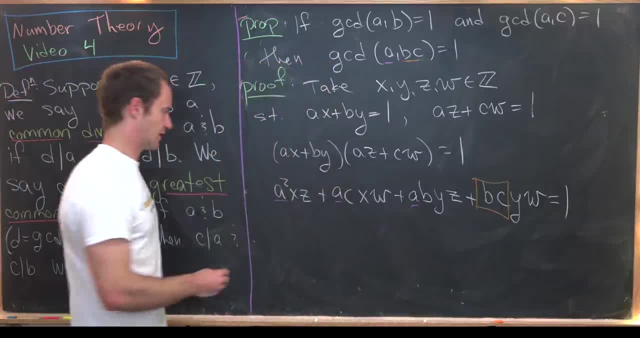 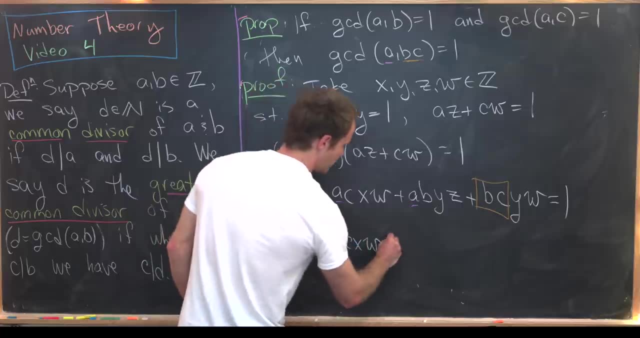 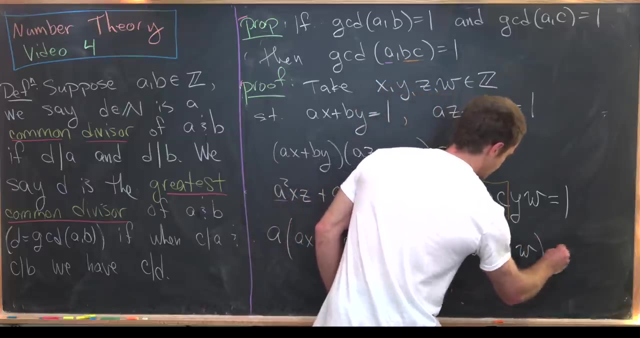 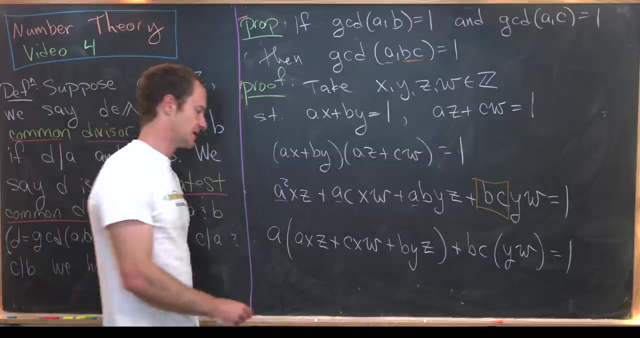 a, So let's maybe factor out accordingly. So here we have a times axz plus cxw plus byz plus bc times yz plus bc times yz plus bc times yz. So we've written 1 as a linear combination of a with bc. but that condition implies that 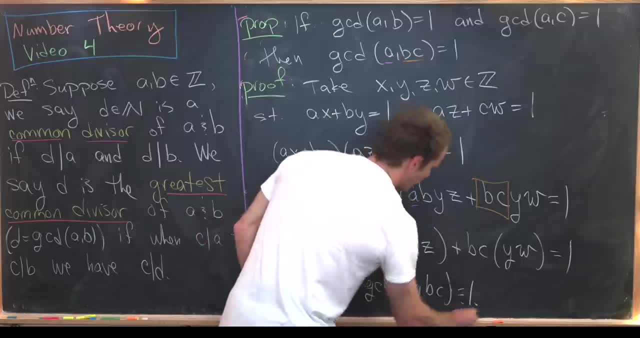 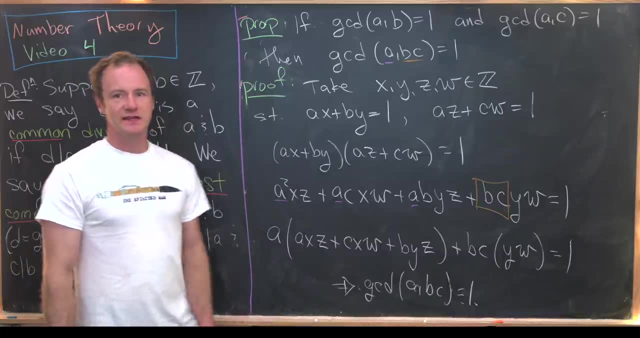 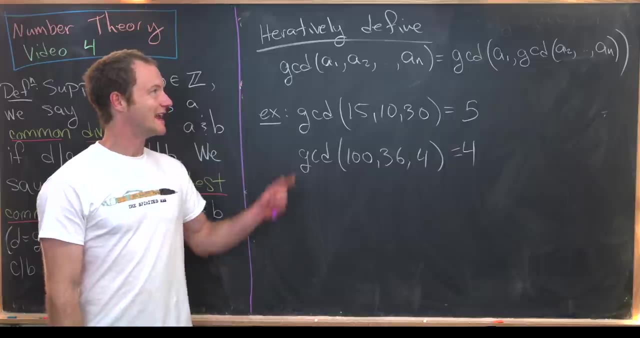 the gcd of a with bc is equal to 1 by the corollary that we just discussed. Okay, so this is our last proposition. Now let's look at an extension of the greatest common divisor to more than two entries. Okay, So we can iteratively define the gcd of more than two numbers. 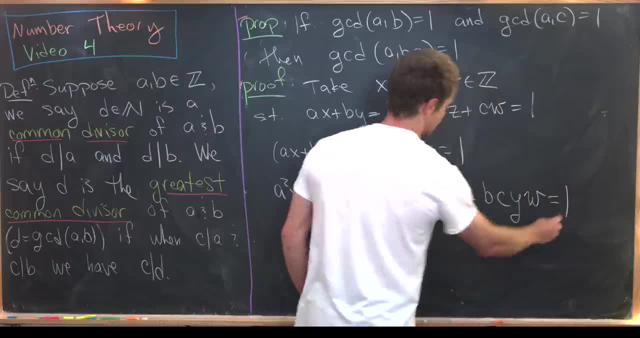 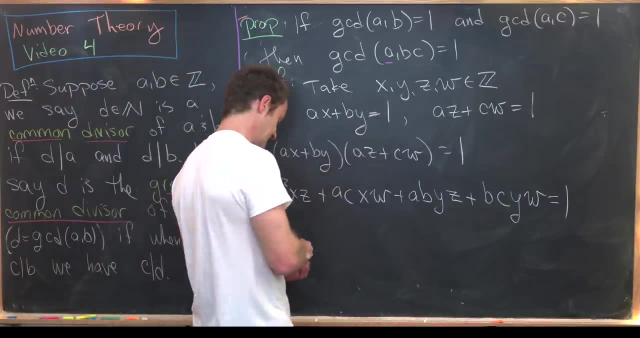 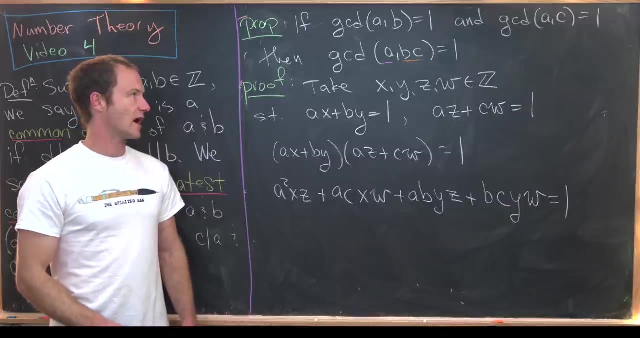 BC times YW equals 1.. But now let's look at what our goal is. Our goal is to show that the GCD of A with BC is equal to 1.. But we can do that if we can write a linear combination of A and BC. 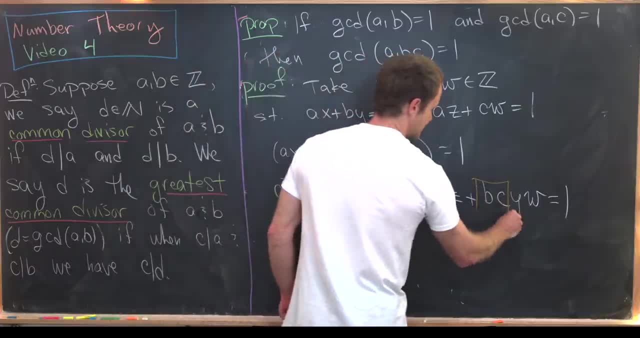 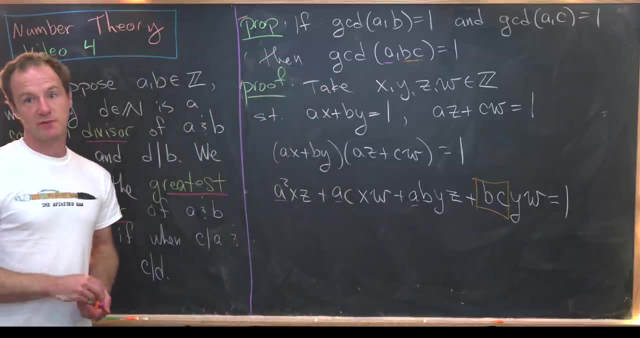 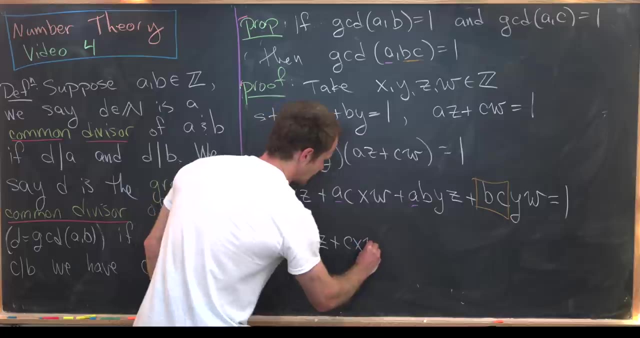 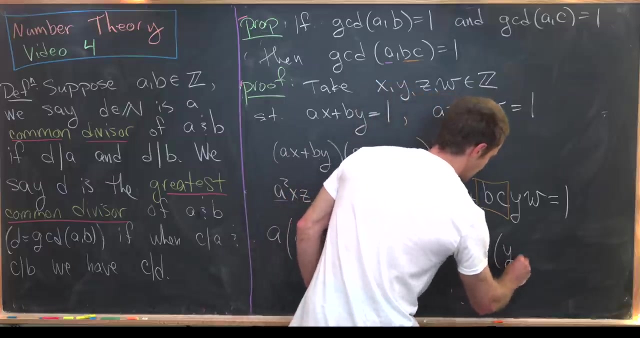 is equal to 1.. We'll notice: here we've got BC and then in all of the rest of these terms we have A, So let's maybe factor out accordingly. So here we have A: times AXZ plus CXW plus BYZ plus BC times, YW is equal to 1.. So we've written 1 as a linear combination. 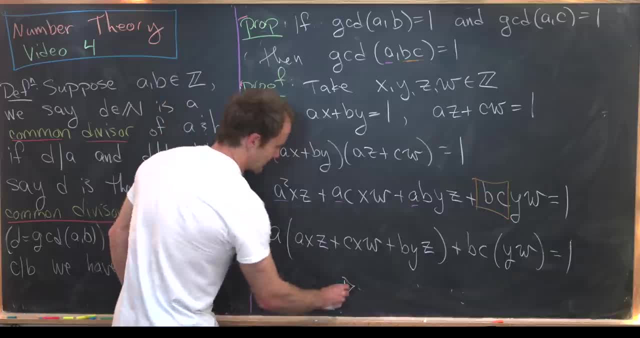 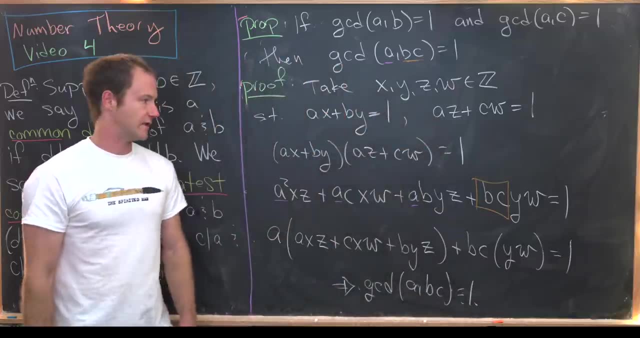 of A with BC, But that condition implies that the GCD of A with BC is equal to 1 by the corollary that we just discussed. Okay, so that's the GCD of A with BC. We can do that if we can write a linear. 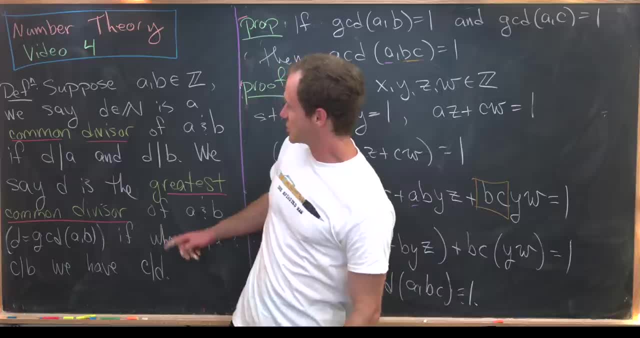 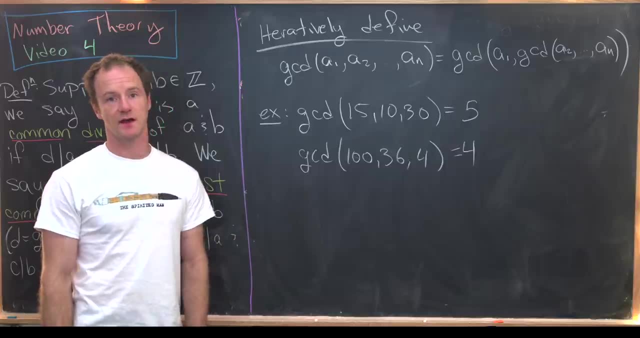 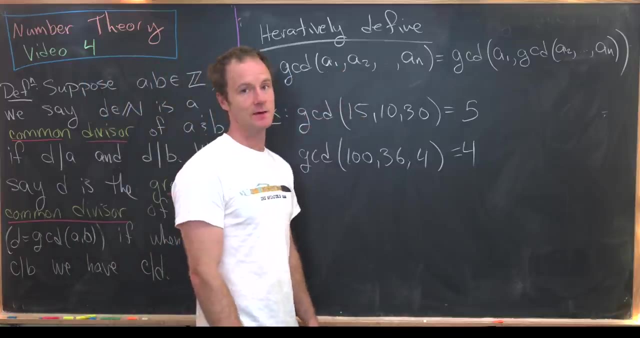 combination of A with BC. Now let's look at an extension of the greatest common divisor to more than two entries. Okay, so we can iteratively define the GCD of more than two numbers. So we can do it like this: The GCD of A1, A2 up to AN is equal to the GCD of A1. 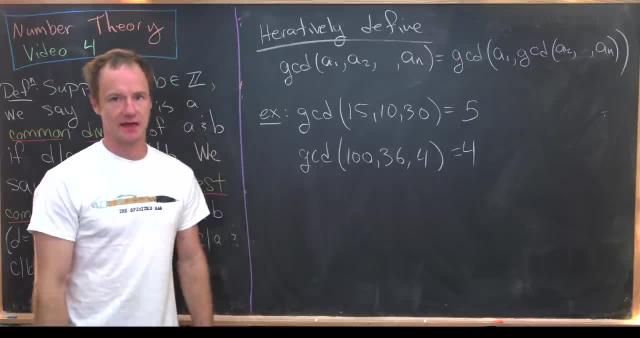 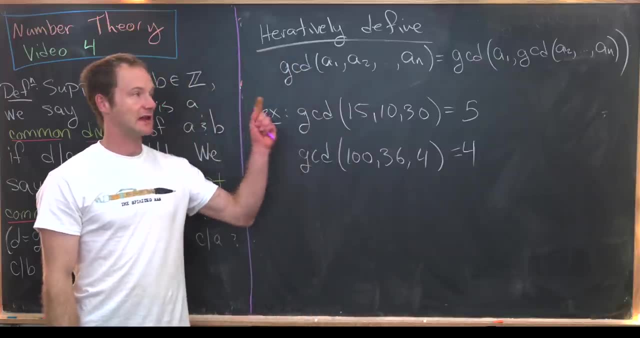 with the GCD of A2 up to AN. So notice, here we're really just taking the GCD of two numbers, A1 and that other GCD, So you can layer these GCDs on top of each other. So let's look at two. 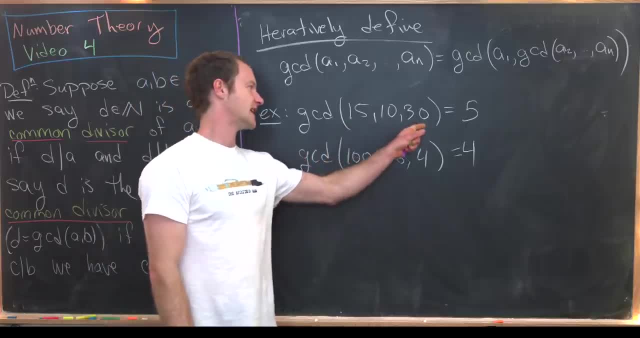 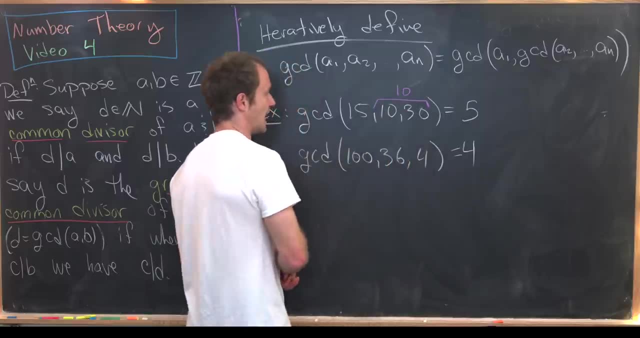 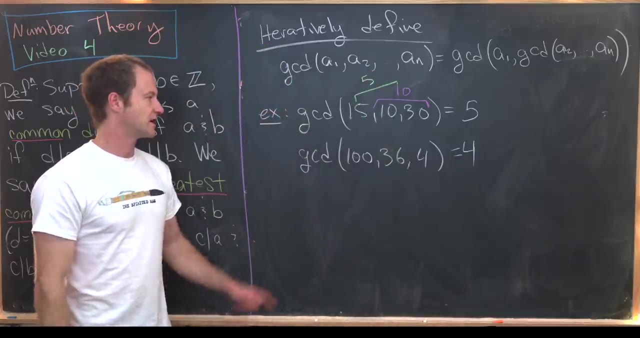 quick examples. So the GCD of 15,, 10, and 30 is 5.. And that's because the GCD of 10 and 30 is 10.. And then the GCD of 15 and 10 is clearly 5.. And then, through a similar argument, the GCD of 100,. 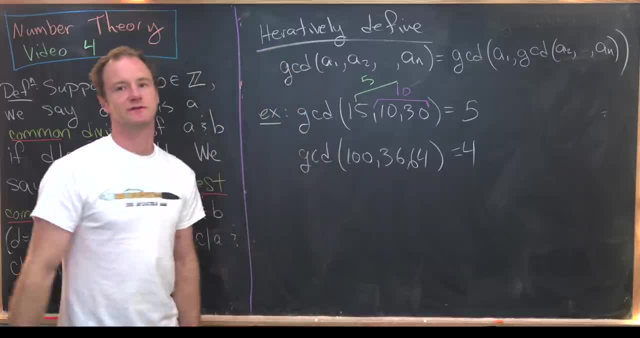 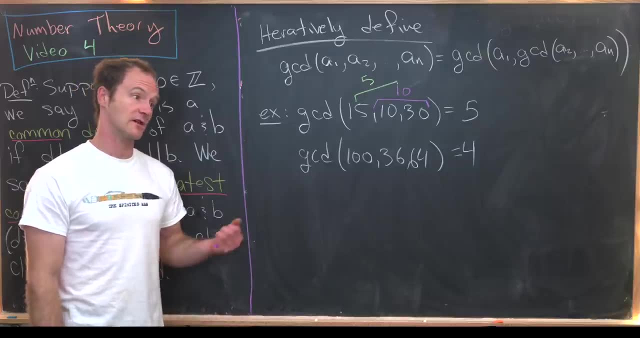 34, and 70.. 64 is equal to 4.. Okay, great. Well, let's finish this video off with some warm-up problems to do before class if you're in my class and maybe just for fun if you're not. 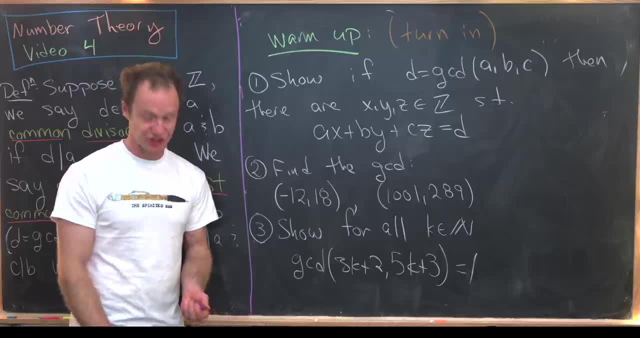 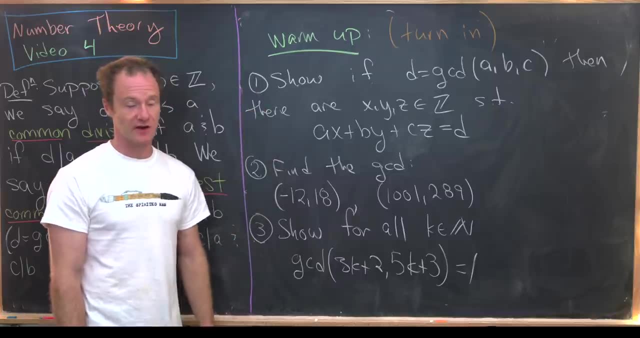 So we'll finish this video with a couple of warm-up problems that are to turn in at the beginning of the next class, if you're in my course. So the first one is really an extension of that first theorem we proved. So let's show that if D is equal to the GCD of A, B and C,